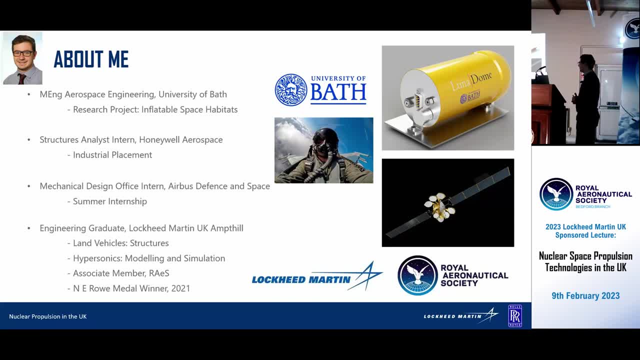 aircraft. So I was a structures analyst so I worked on stress analysis for those pneumatic systems. so it's taking bleed air from the compressor in the engine, passing it through valves, heat exchangers, rotating compressor, turbine assemblies, water separators, things like that to pressurize the cockpit and cabin and also provide oxygen for. 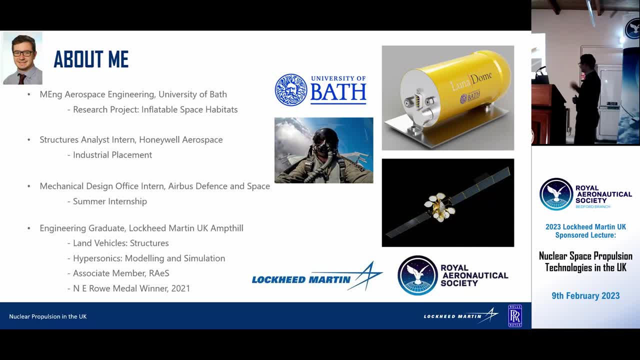 the fighter pilot themselves. Once I returned back to uni I realized aerospace was for me, so I transferred to aerospace engineering, did a couple of years in that and, as part of what I learnt during my industrial placement, I actually entered a competition in my third year which was run by an. 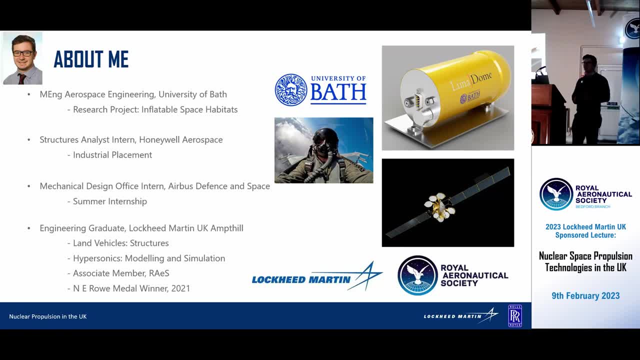 Indian company called Team Indus and they were creating a lunar lander as part of the Google Lunar XPRIZE to land a rover lunar lander on the moon, deploy a rover, take pictures, send it back to Earth and as part of that program they set up a competition called Lab to Moon, which was a 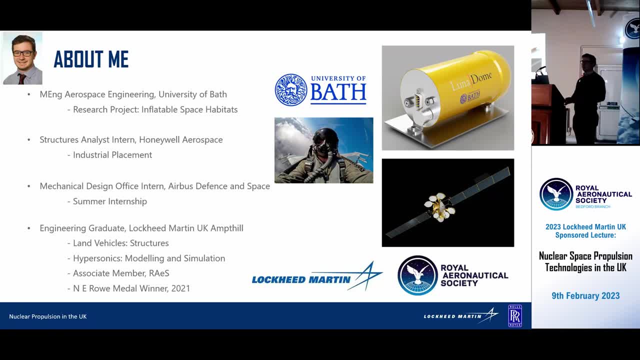 student competition to create a payload for their lunar lander and do some useful science. So my project was called Lunar Dome. it was an inflatable habitat that is the size of a soda can and it inflates a flexible material so atmospheric pressure maintains it for as long as possible. So 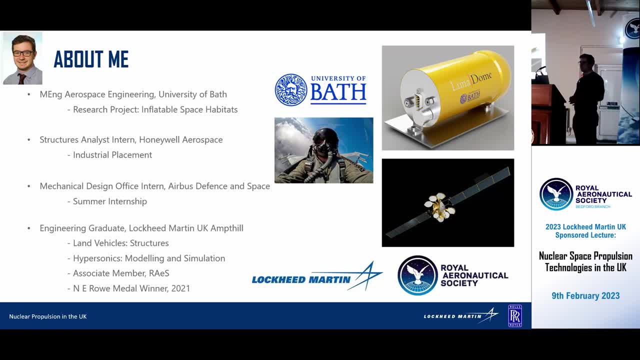 yeah, we entered the competition. there was 3,000 entries and we ended up coming third. so we got a contract to put the experiment on the lunar lander and, yeah, the rest is history. So I'm looking forward to working with you guys in the future and I hope to see you in the future as well. 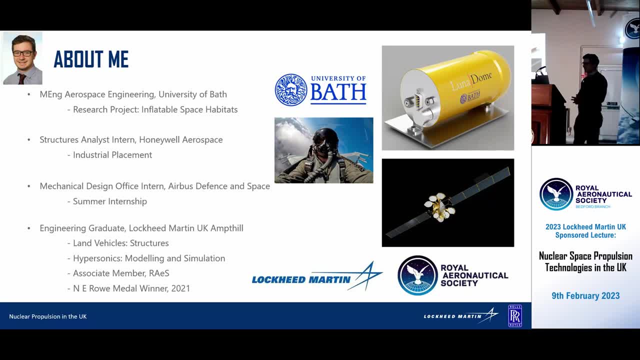 Yeah, after I left my fourth year at uni, I did a summer internship at Airbus Defence and Space in Portsmouth. So they manufacture large telecom satellites for civil and military applications. So I was working in the mechanical design office working on design of the payloads that go onto the 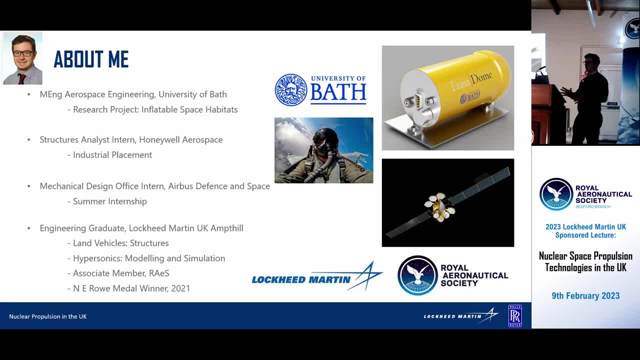 satellites, also looking at stress and thermal analysis, looking at launch conditions and then in service conditions, trying to make sure that everything can be signed off and put onto those large satellites. Once I left uni I joined Lockheed Martin, so I started as a graduate engineer. 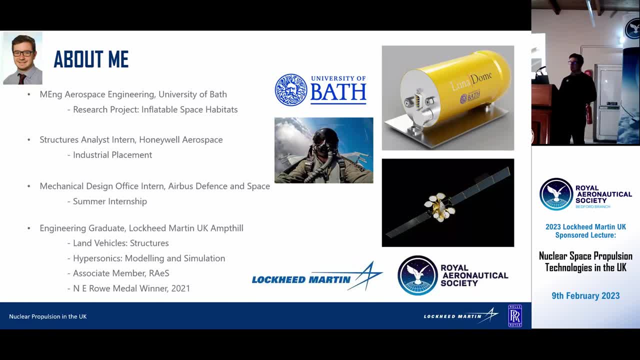 did that for two years, rotating around the business. There's quite a wide variety of different roles you can do, so I started off in land vehicles, did a couple of rotations there and then moved to the more aerodynamic side of things- modelling, simulation- which is kind of what. 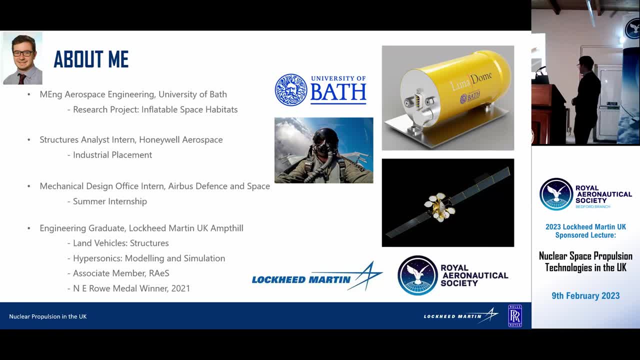 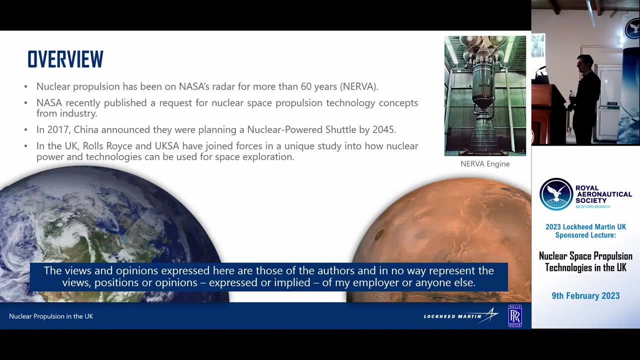 I do now. I've been an associate member of the Royal Aero Society for a couple of years now, and through that I have won that NE Roe medal. So that's pretty much me. So a bit of a disclaimer to start with. we always have to do these as part of these. 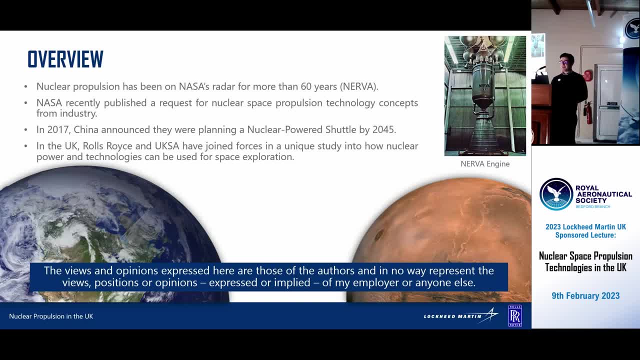 presentations. So the views and opinions expressed here are those of the authors and in no way represent the views, positions or opinions expressed or implied of my employer or anyone else. So getting onto the meat of the presentation, so nuclear propulsion- A lot of people don't know that. 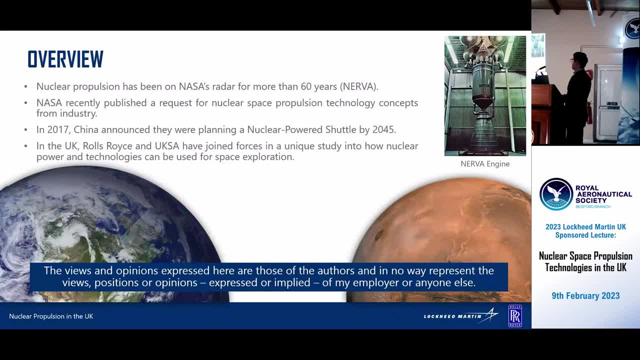 nuclear propulsion for space applications has been around for a long time. NASA started investigating nuclear propulsion in the 1950s to 1960s. Their kind of flagship program was called the NERVA, so the nuclear engine for rocket vehicle applications. 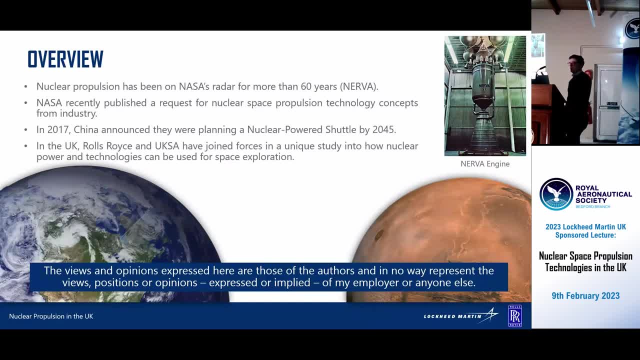 And this was kind of a test program where they put hardware on the ground. So they used a hydrogen fuel source, passed it through a reactor for a converging diver to measure efficiencies, thrust and all sorts of different parameters. So the kind of basis for this study was a couple of things. 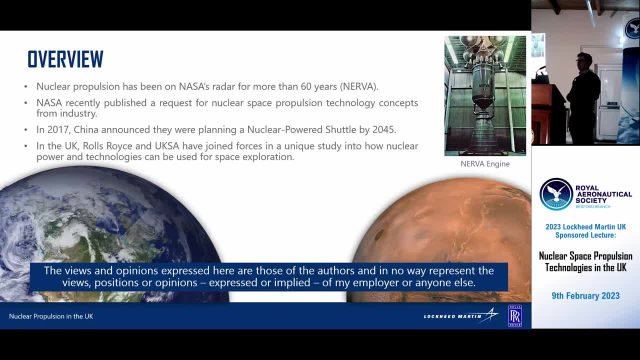 So NASA in 2021 published a request for industry to develop nuclear space propulsion technologies. So that's nuclear thermal propulsion and nuclear electric propulsion, which I'll get into more detail a bit later. So that came out in 2021.. There's been a load of contracts that have been given out since then. 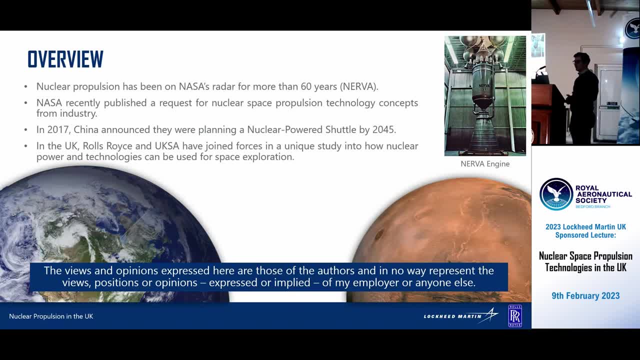 And recently there's been a lot of investment in there In the past couple of months. elsewhere in the world, China have announced that they're planning to produce a nuclear powered space shuttle by 2045.. And the real meat of this presentation is about Rolls-Royce and their development. 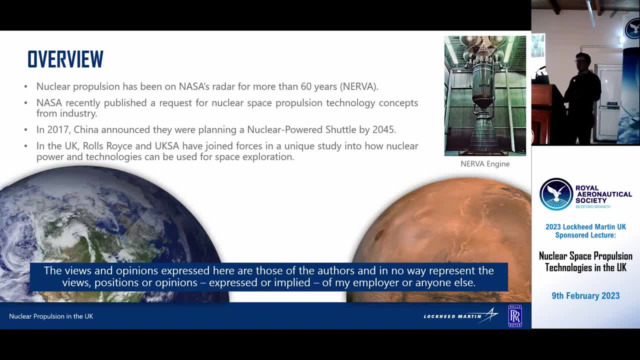 So in 2021, they produced a kind of roadmap for the UK to expand their technologies within the space industry. So I think at the moment the UK takes about 4% of the space industry globally And by 2030, they want to expand that to 10%. 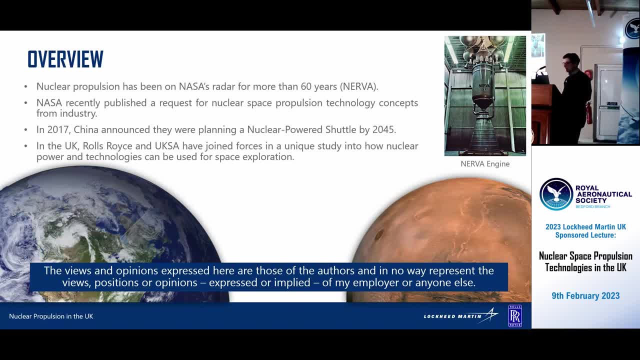 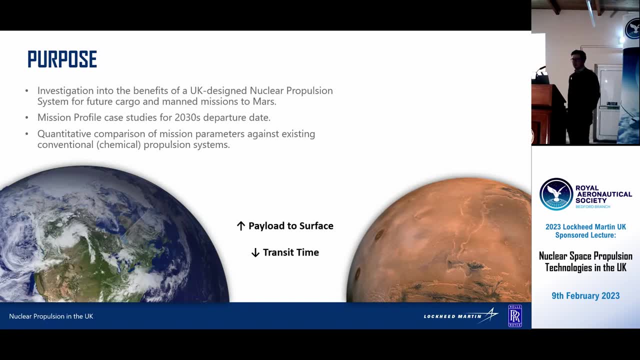 And Rolls-Royce are going to be a big player in that, especially on the nuclear side of things. Okay, so, purpose of this study? So, as part of the project on nuclear issues conference that we presented in, we get a chunk of hours to do a kind of standalone study, to assess something, write a presentation. 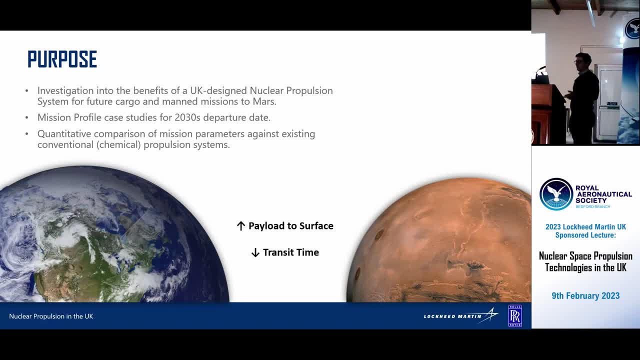 then write a paper on it. So what we decided to do was investigate A comparison between conventional propulsion systems and nuclear propulsion systems in transporting both cargo and people from Earth to Mars, Looked into mission profiles around the mid 2030s And we were kind of comparing two kind of major quantitative values, measures of how. 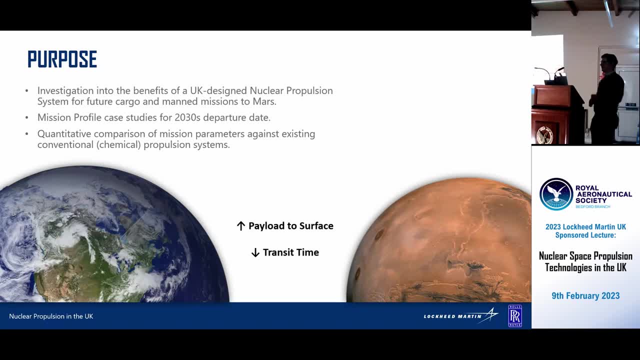 good a system is. So with cargo missions, Obviously you want to transport as much payload as possible to the surface. Once you're there you can. then, if you've got a lot of mass there, you can bring a lot of science equipment, bring building materials, tools to create a habitat, create a base. 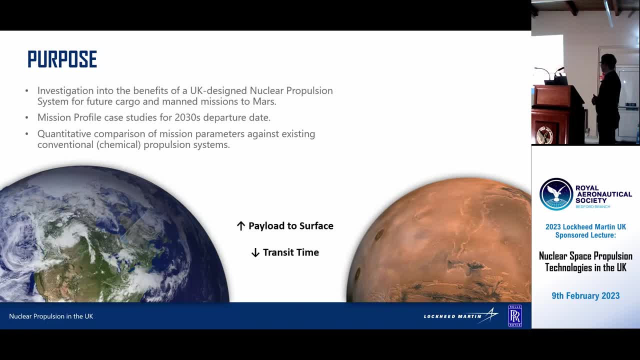 create infrastructure, things like that. So you want to maximize the payload to surface in the cargo missions. In the manned missions we want to minimize transport time. So that's for two reasons: One is to reduce the payload to the surface. Two is to reduce the passengers exposure to cosmic radiation, microgravity effects. which can affect your sort of bone density, your muscle loss, et cetera. Also because transfer times typically take in the order of six, six to seven months. So who wants to be in a spacecraft for six to seven months? Definitely not me. 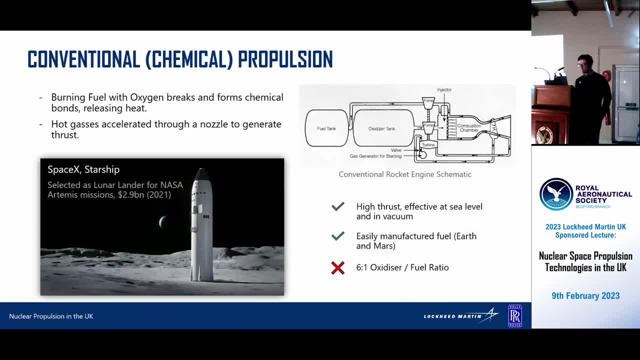 So trying to minimize that is beneficial. So next question: I'm going to ask you a question. I'm going to ask you a question. Okay, So I've got a few slides. I'm just going to go through kind of a basic overview of different types of propulsion. 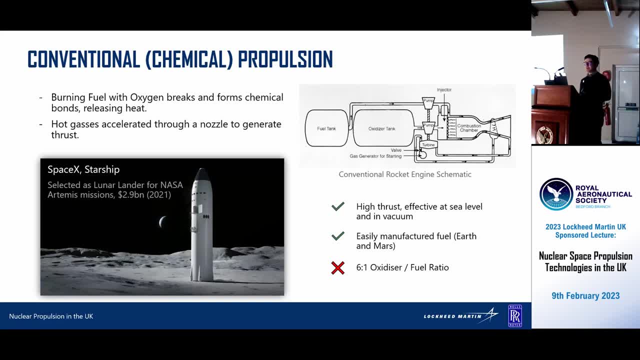 systems. So starting with sort of chemical, conventional liquid powered rockets, So on the top right we've got two different tanks: or your fuel tank, which typically contains combustible materials such as liquid hydrogen or something like kerosene, RP1,, if you know. 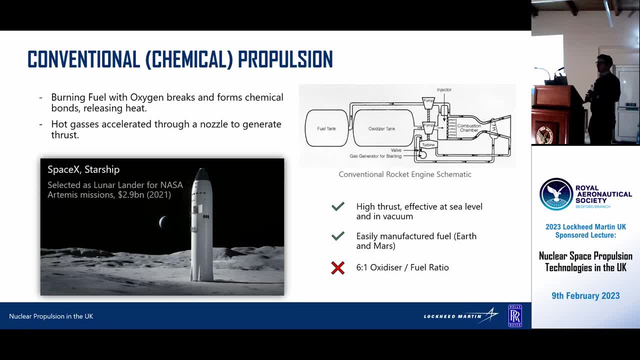 about rocket fuels. And then you've got an oxidizer tank which is pretty much solely there to initiate the combustion and maintain the combustion process. So typically that's liquid oxygen. So benefits of these systems: you get very high thrust, So they're effective at both sea level and in a vacuum. 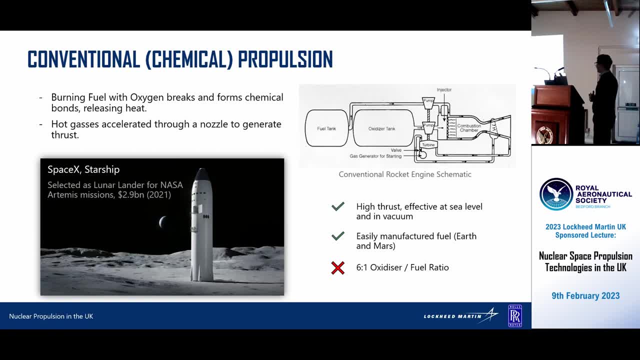 So, depending on your configuration of your nozzle, you can have your first stage to launch the rocket off earth Using a nozzle that's configured. So you can have your first stage to launch the rocket off earth using a nozzle that's configured, That's configured specifically to work in the atmosphere. 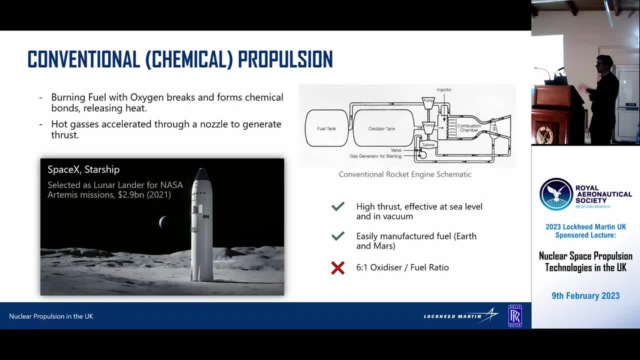 And then you've got your second stage typically has a slightly different nozzle which is configured to work in a vacuum. So the way you sort of this kind of flow is: you've got your two liquid propellants. They flow through the pipework that's in the system, goes through a couple of turbo pumps. 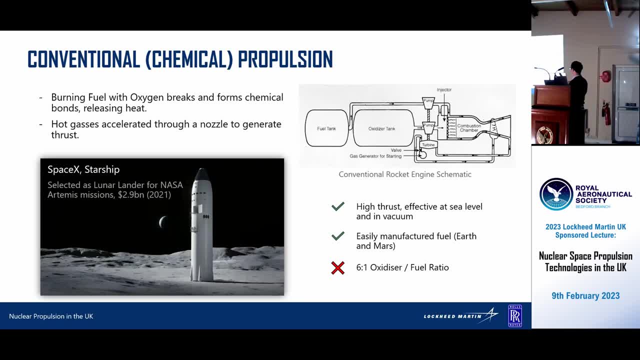 to increase the pressure as it goes into the combustion chamber. Once it's in the combustion chamber, The gases combine, the combustion process is initiated and maintained, and then it flows through a converging, diverging nozzle to convert thermal energy and pressure into velocity. 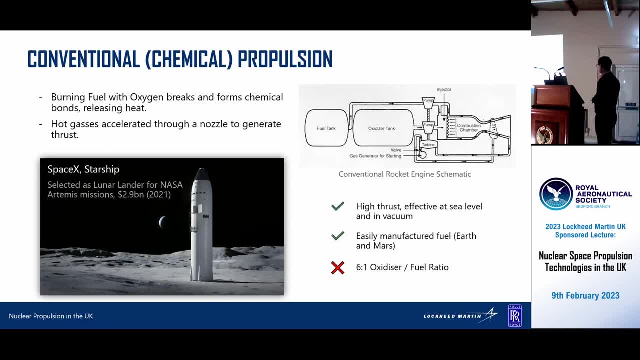 which is then reacted back through the rocket. So another benefit of this, these types of systems, is, once you actually get to Mars, the fuels that you use are actually quite easily manufacturable. So both on Earth and Mars. So with this example, I've got here the SpaceX Starship. they use methane and oxygen and 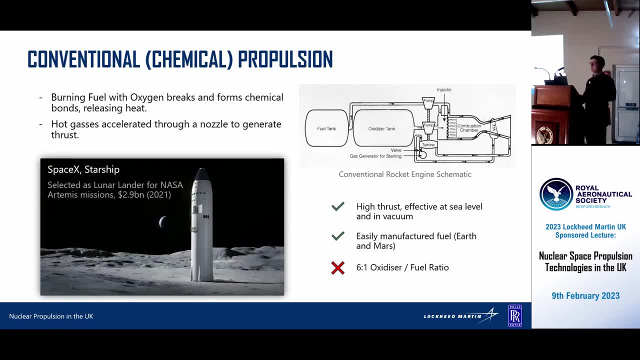 there's quite simple chemical processes on both planets to be able to produce both fuels. So, yeah, it's beneficial to be able to use those. Major downside, of course, is you've got a useful fuel tank and pretty, almost redundant oxygen that you're using. 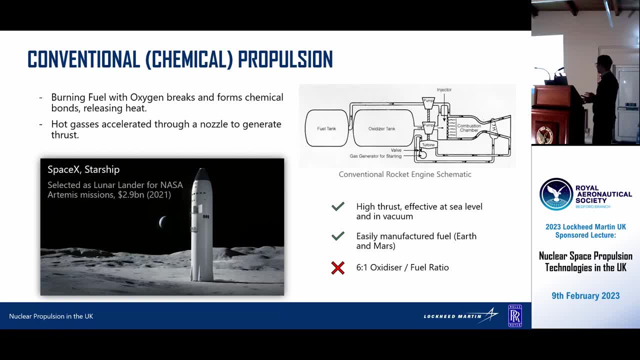 So you normally have a six to one ratio, Yeah, Between the masses of each. So ideally if you could remove the oxidizer tank and remove the oxidizer that's in it, you can replace that with useful payload. So example: I've got on there of a contract that's recently been awarded to SpaceX. 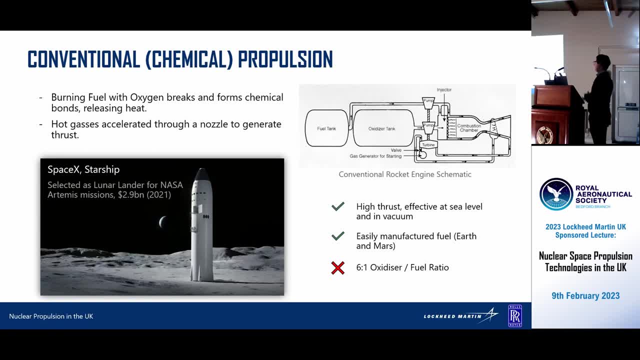 So I think yeah. 2021, NASA awarded them a massive three billion dollar contract to develop the Starship to carry human To the moon as part of the Artemis missions, and in the future they might be developing that into going to Mars as well. 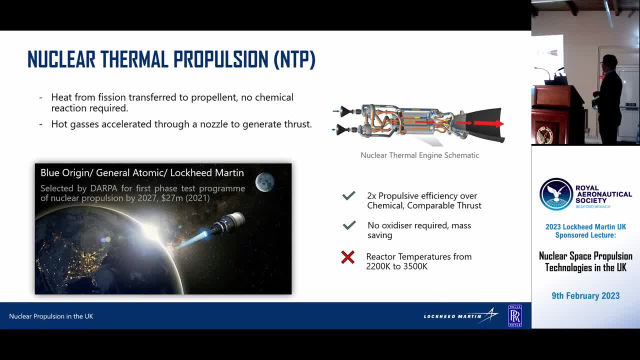 So getting on to the nuclear side of things, So it's two different types, two main types. So the first is nuclear thermal propulsion and essentially it works in a similar way to the conventional case, except you've only got one fuel. So typically you use hydrogen and you pass hydrogen through a similar kind of pipe work. 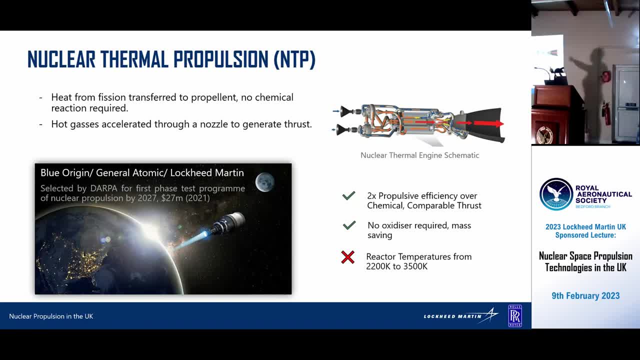 and then the main difference is that you've got a reactor, a nuclear reactor, instead of a combustion chamber, And the nuclear reactor generates heat, transfers that to, And then again it's expanded through a converging, diverging nozzle to produce thrust. 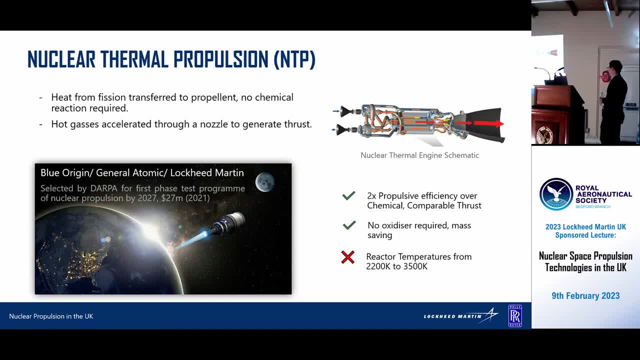 Compared to conventional systems. no oxidizer is required, So there's no oxygen there in the process at all. So, as I mentioned, Yeah, Yeah, huge mass saving which can be replaced with useful payload. but then a huge downside is, despite the fact that you're transferring heat from the reactor to the fuel, you still transfer. 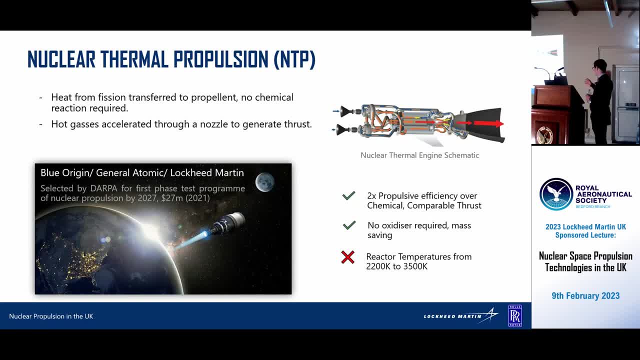 a lot of heat to the surrounding structure as well. so you get reactor temperatures in the order of thousands of kelvin and you need to do something with that heat. so you kind of need to design some quite complex cooling systems for the structure to ensure that everything. 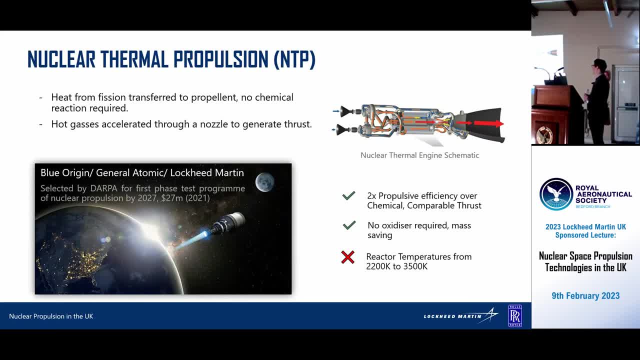 stays intact, i guess. so yeah, example: i've got there a recent contract that's been awarded by DARPA to blue atomic and lucky martin in the us to design a nuclear thermal propulsion system which i believe is planned to be flight tested around in earth orbit by 2027. 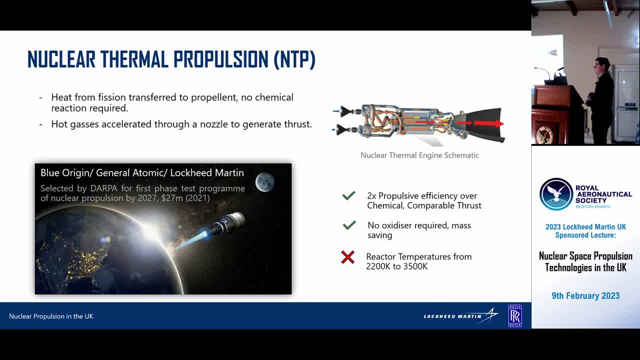 it's a 27 million dollar contract, but i think last week nasa has announced that they're going to be joining forces with DARPA in this contract and they're going to be plowing a lot more money into this development. so i think it's an undefined amount of money at the moment, but 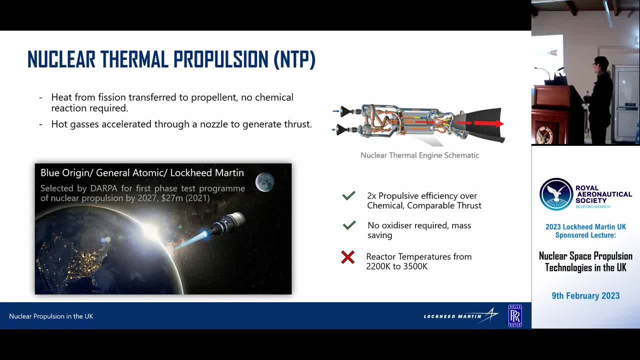 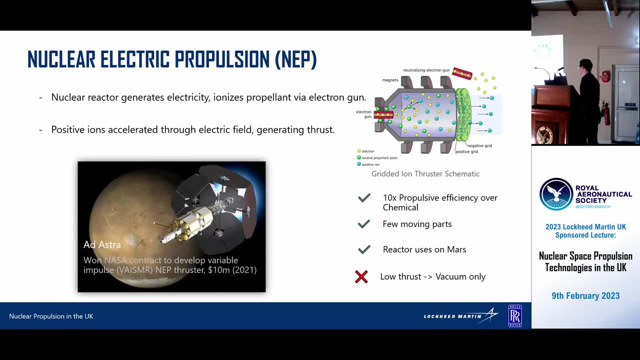 guessing it's going to be comparable to the, to the ones we see with spacex. so finally, nuclear electric propulsion. so the main difference here is you're, instead of using the nuclear propulsion, you're going to be using the nuclear propulsion reactor as a heat transfer source. you use it as an electricity generator. so the way, the thruster, 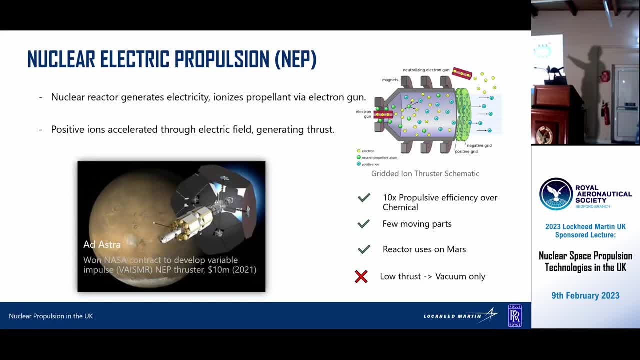 works is you start with the electricity coming off. the reactor comes through an electron gun, so you've got electrons being fired up. then you've got fuel coming around the outside of it and coming into the thruster as well. typically these fuels are, you know, it's gases such as xenon or krypton. 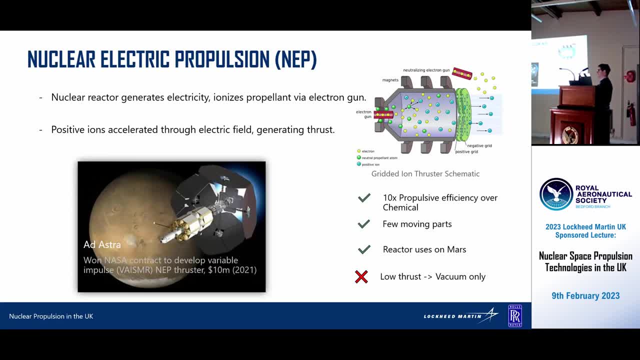 which are much heavier than the nuclear reactor. you can't really do that without a fuel, so the much heavier than hydrogen or methane. there's typical fuels for the other two systems. so once the gas gets into the thruster the electrons collide with the atoms in there and they knock off electrons from those atoms to ionize. 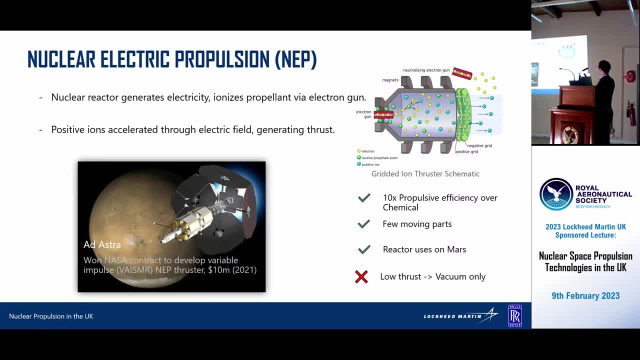 them and then those ions are accelerated through a magnetic field and an electric field to really really high speeds, so you can get close to relativistic speeds- around 10% the speed of this, the speed of light- and then they're rejected out of the thruster and there's a secondary neutralizing electron going at the top. 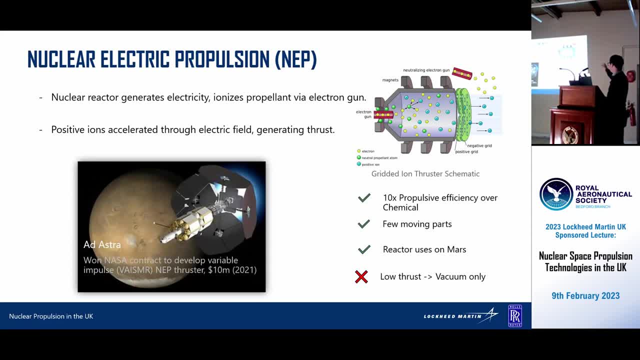 which then fires additional electrons back at the ions to neutralize their charge. that's the way that produces thrust. so typically you get a huge amount more efficiency from these thrusters, so ten times more than chemical energy. so there's a huge benefit is there's very few moving parts, so it's a. 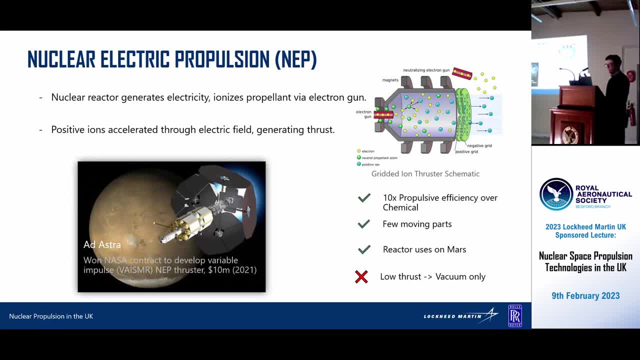 mechanical engineer's dream. very simple to design from a mechanical perspective. but you get really good reactor uses on Mars. so because you're generating electricity with your nuclear reactor, you can essentially use that reactor to produce electricity once you actually arrive at Mars. so when you're producing 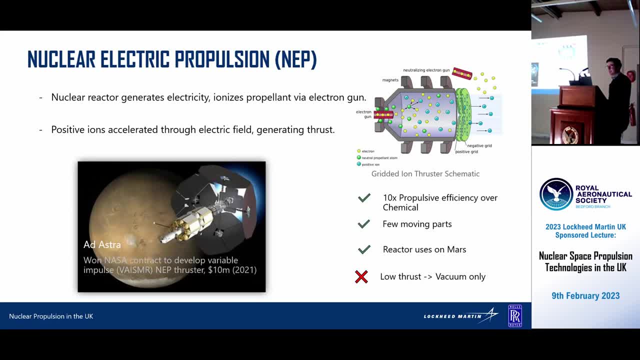 your base that you can use that useful energy there. so typically I think reactors have lifetimes of around ten years, so once you actually arrive on Mars, you've still got a huge amount of useful energy that you can use to use up. the downside it's very low thrust, so typically you have to use these engines for in the order of: 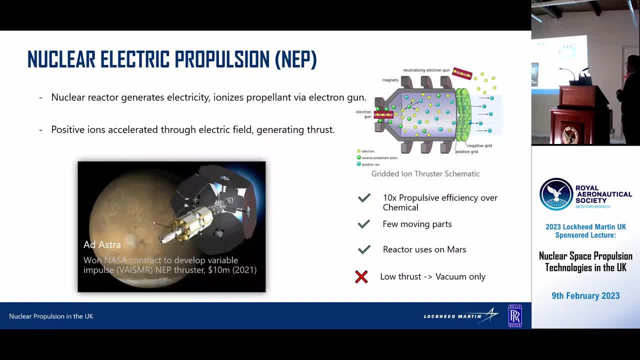 weeks or months, so when you're traveling through space you have to have them on for a very long period of time to have any kind of meaningful velocity change of your spacecraft, which means that they're only really useful in vacuums, so you can't use them to launch from the earth. 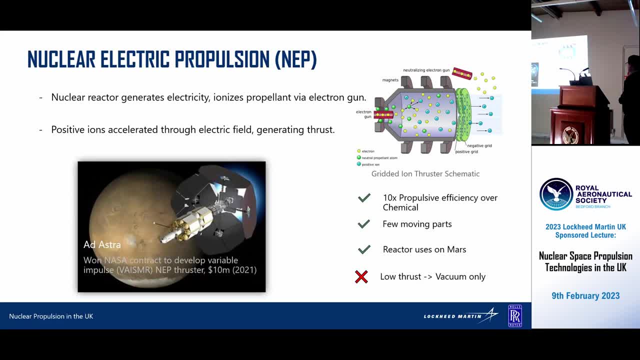 surface and escape the gravity field. so that means they kind of have to be used in conjunction with the other two, one of the other two propulsion systems, so chemical or nuclear, thermal, to escape earth. then in your second stage, when you're하�άνَا. 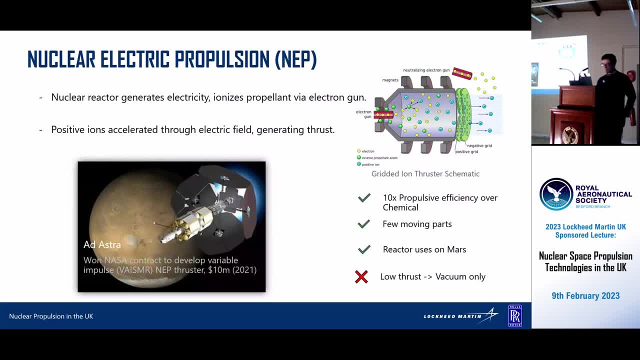 a vacuum. you can then use these to their full potential. so i've got a example of a another contract which was awarded a few years ago to add astra to develop a variable impulse nuclear electric thruster. it's a bit smaller contract this time, 10 million dollars, the kind of announcement. 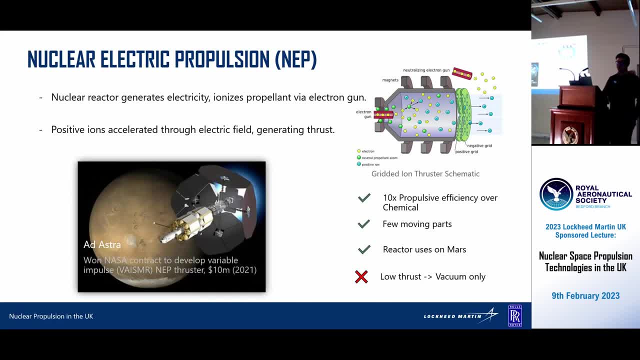 that i mentioned in the last slide, where nasa are joining forces with darpa. so not only are they investing in nuclear thermal propulsion, they're also plowing a lot of money into this technology, and this is the technology that rolls-royce are really interested in as well. 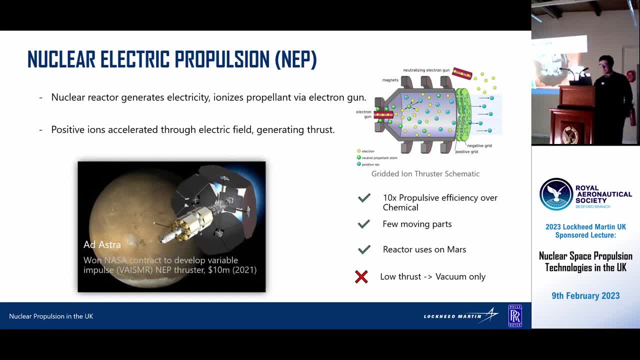 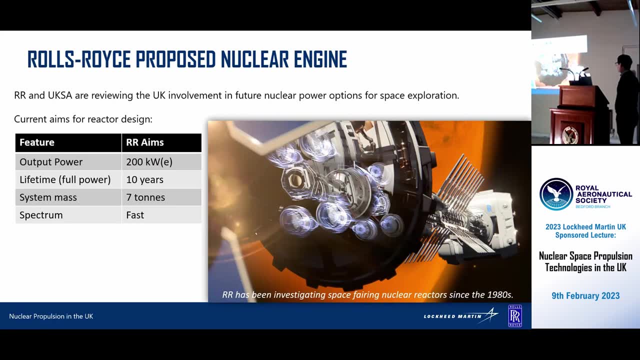 so that was kind of a big focus for us. so, as i mentioned, roles in the uk space agency are reviewing the uk's future in the space industry, trying to lay out a roadmap for us to expand our market cap. so not only are they designing reactors, they're also designing spacecraft structures and systems. so in this example, 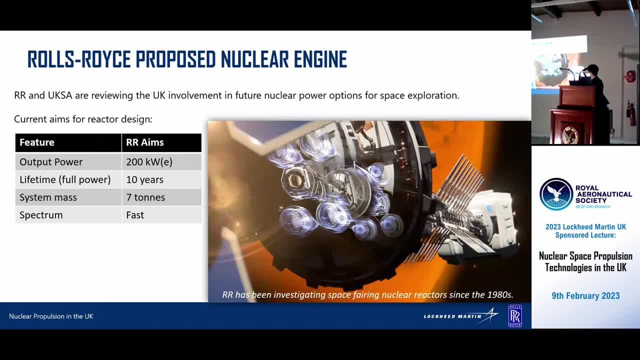 the thrusters are on the left-hand side there and the crew and passenger compartment is way down on the other side of the spacecraft. so the reason for that is for safety reasons. so you don't really want your humans to be close to your reactor. so separation is really useful in reducing the 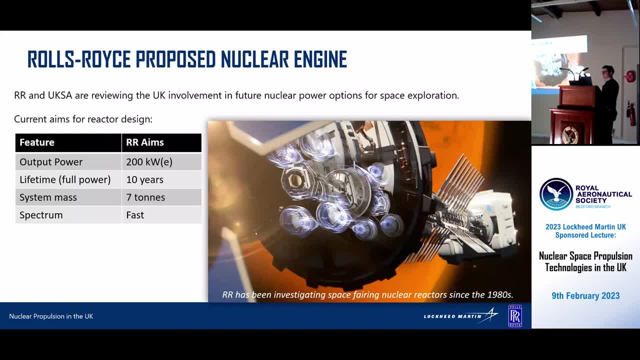 radiation dose. you can also put your fuels in between your reactor and your passengers so that attenuates a lot of the radiation coming through as well, and then also you can use discs fields, so you can see these two black shields there, which are kind of high density material that can also reduce. 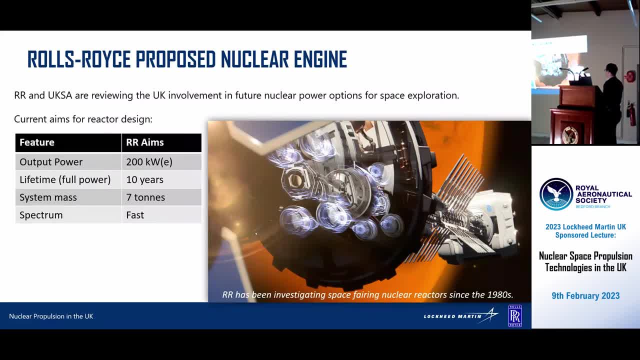 radiation exposed to the crew and then that long boom. you can see in between the two example of how elaborate your cooling system has to be. so if you've seen pictures of the space station, you'll see a load of radiators coming out of it, and this is a similar thing. 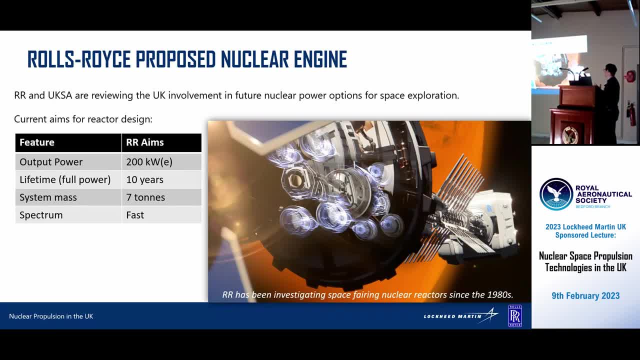 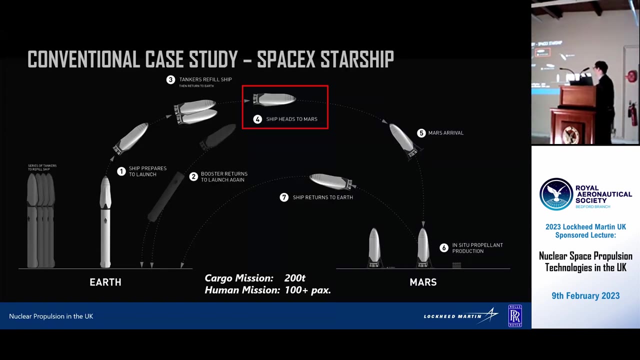 where we're trying to cool down our reactor and project a lot of that heat as radiation into space. so there's a lot that needs to go into actual spacecraft design. we're thinking about these propulsion systems. so going into a bit of the analysis of what we actually did in this study, so we started off with a 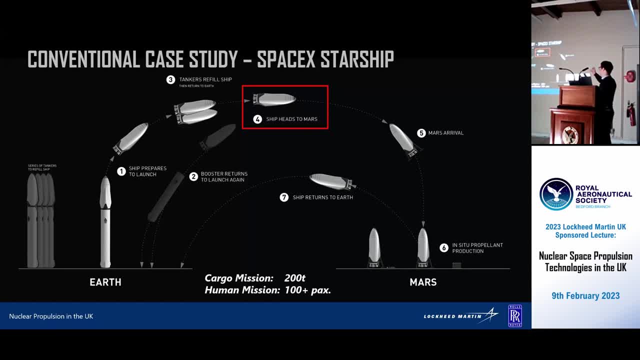 looking at a case study of the Starship. So SpaceX is looking to transport masses of humans from Earth to Mars. It's going to be a reusable spacecraft, so they're going to be looked at and all of the structure is going to be reusable. So working through this kind of mission profile. 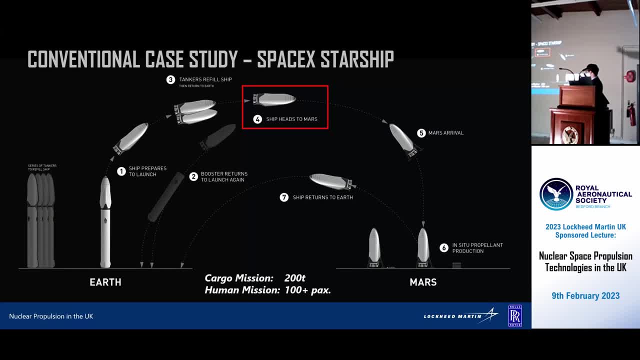 we start off step one. So we've got a booster and Starship attached to the top of it which is filled with passengers. The booster will launch into Earth orbit and it will stay there for a while. Alongside that we'll have fuel tankers that will launch, so it'll be boosters. 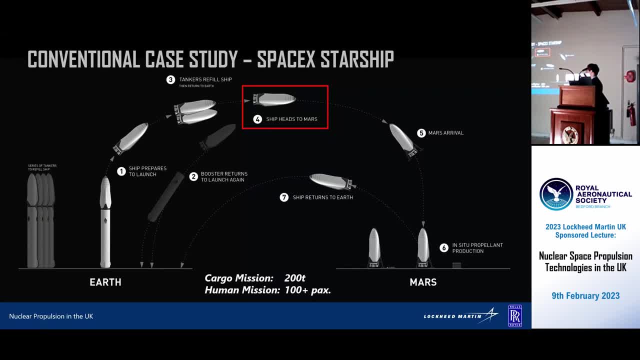 with a spacecraft that contains fuel as payload. They will launch into Earth orbit at the same time. They'll then perform orbital refueling around the Earth, and then the boosters, obviously, when they separate, they'll return back Once the Starship, which contains passengers, is then fully loaded with fuel. we then look. 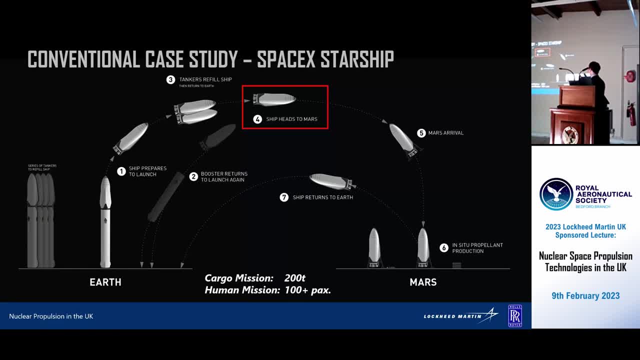 at step four: your long duration- transport to Mars. So step four typically takes six months. It's longest duration, longest amount of intensity on your engines, your fuel burn. So that's kind of the step that we're most interested in. That's the step you can get. 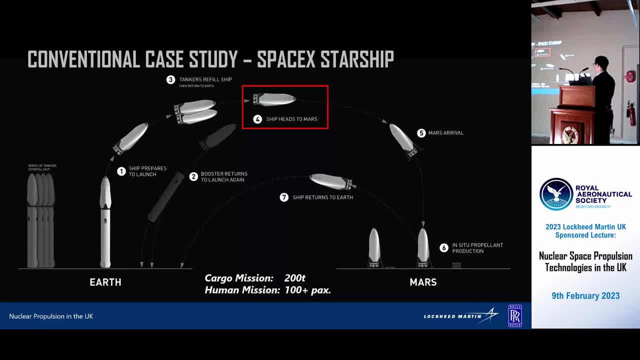 the most benefit out of using nuclear propulsion systems. So once you've arrived at Mars, then perform a landing burn. You'll land on Mars, you will perform your mission And, as I mentioned earlier, it's quite easy to produce fuels once you actually get to Mars, So you can do in situ propellant production. All this time we're 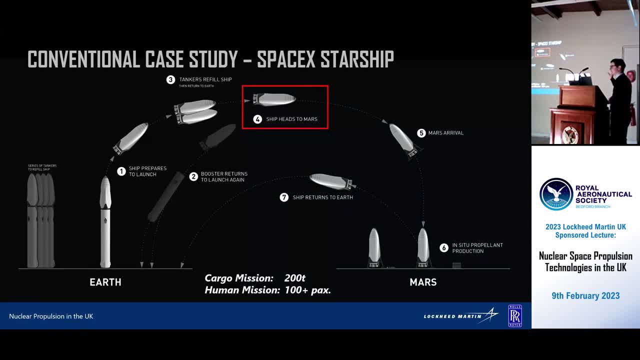 going to have more and more ships landing, Build up for people got the amount of infrastructure structure. once we have good production facility fuel, we'll then be able to refuel our spacecraft, return back to earth and then redo the whole process. so, as i've said, step number four is the 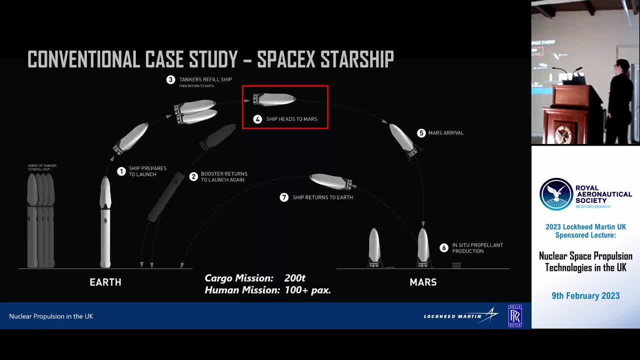 most interested, most interesting from a nuclear propulsion perspective. so that's the step we looked into as part of this study. so the bottom there we've got our cargo mission and human mission. so this is quite an old diagram. i think it's from 2016, but at that time spacex were. 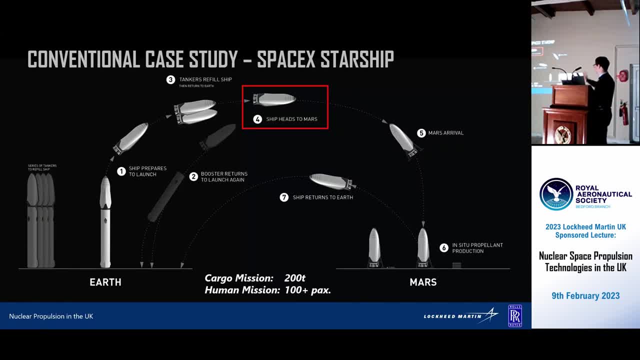 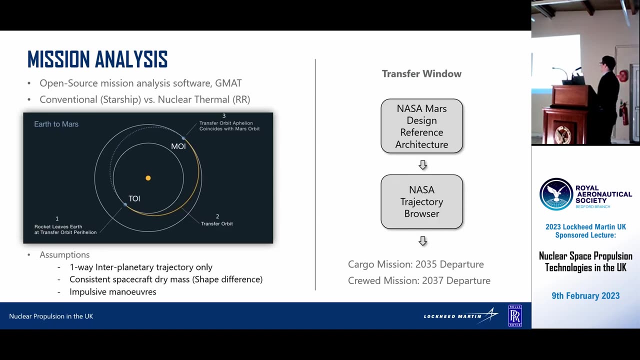 predicting. with a cargo mission you can take 200 tons of useful payload to the surface per mission, and with human rated missions you can take up to 100 passengers. so with all that in mind, kind of used a bit of software that we could estimate the difference between the chemical propulsion system and the nuclear propulsion system to 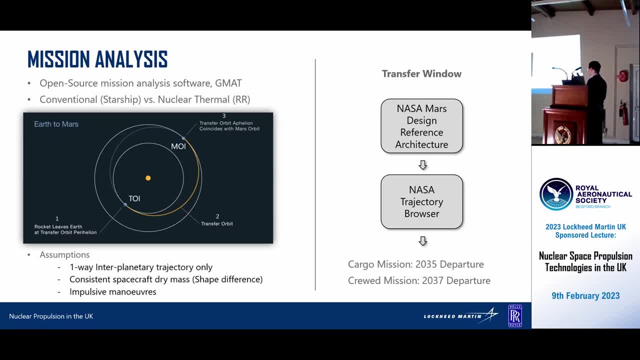 perform a mission to mars on that step four. so we used a bit of software called gmat, open source, and we have one site at lockheed. our assumptions were that we used the starship conventional system and we compared that against the nuclear thermal propulsion system with the. 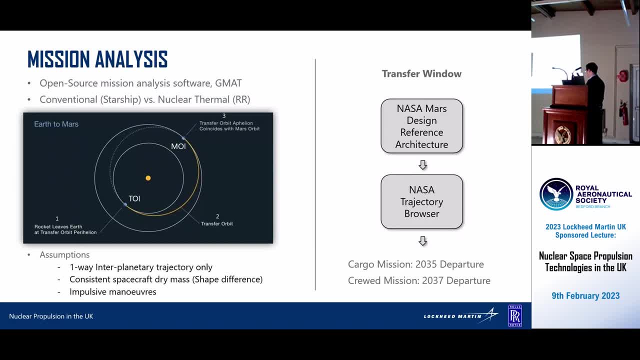 nuclear reactor designed by rolls-royce. further assumptions, and we assumed it was a one-way interplatform trajectory only, essentially the return leg to the same benefits. so we only looked at one way. we assumed that the spacecraft mass, prime mass, with no fuel in it at all- was identical between 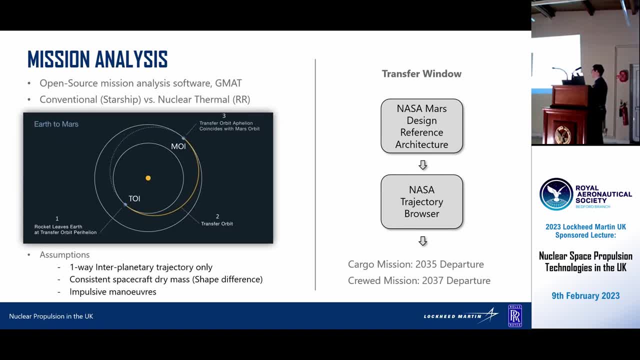 the two systems we're doing knowledge as a shape difference because of all the safety things we're talking about. separating the passengers away from the reactor is quite an important thing to consider. we're working so closely on the 너 you've ring is mars's orbit, so we've got two maneuver points there. we've got toi, which is called a. 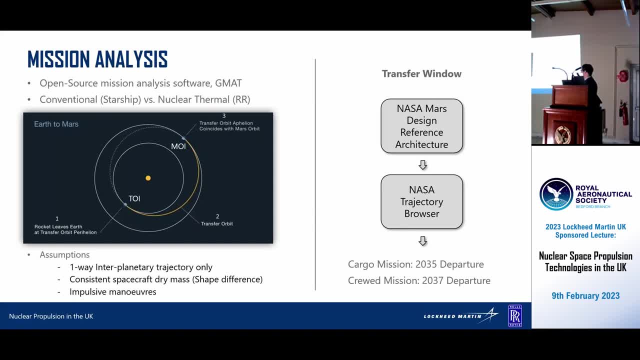 trans orbital insertion. so once you're in earth orbit, you perform a burn to escape earth's gravity and then you go in that orange trajectory towards mars with martian orbital insertion maneuver, where you flip your spacecraft in the other direction, burn your engines to slow down and then you get captured in martian- uh, the martian gravity. well, 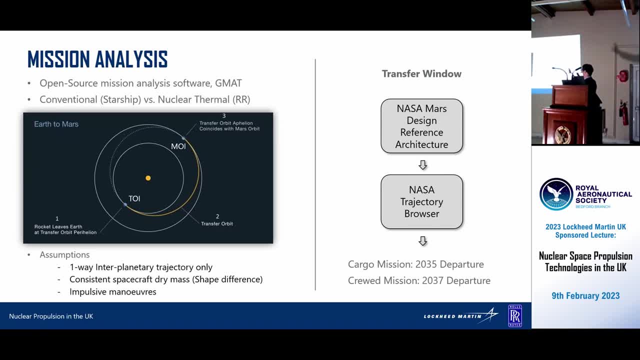 um, yeah, so essentially because obviously earth orbits the sun at different rates to mars, you need to be able to time this transfer really well. so ideally you'd want for earth and mars to be right next to each other, on the same side. so here again, obviously earth rotating around the sun, so 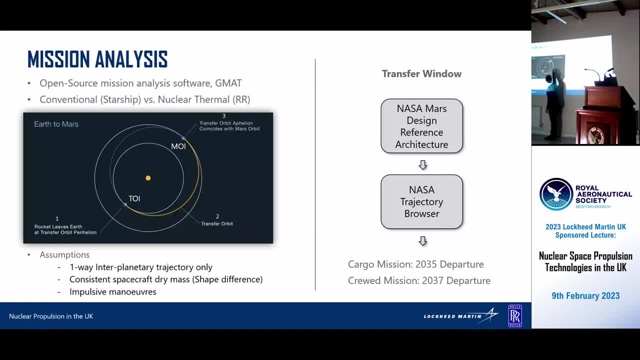 uh, you want to be close, and then they kind of follow each other, get closer and closer to get to that position there. um, that's where, uh, you land. so the way we kind of worked out these timings, um, we use the nasa design reference architecture for mars, which kind of said: 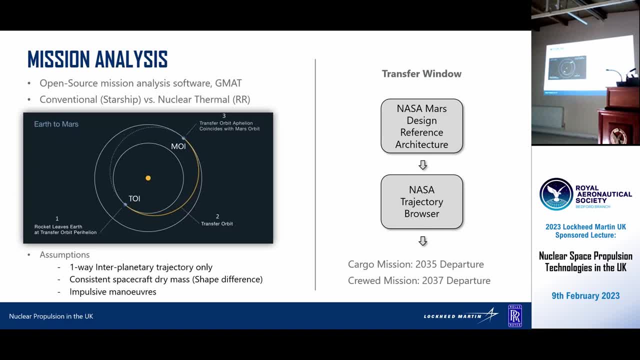 when each technology is available, so roughly in the mid-2030s is a good spot to perform these kind of missions. we then looked at the nasa's trajectory browser, which is an online tool which basically, uh, basically tracks the relevance of earth and mars and it kind of says: what is the? 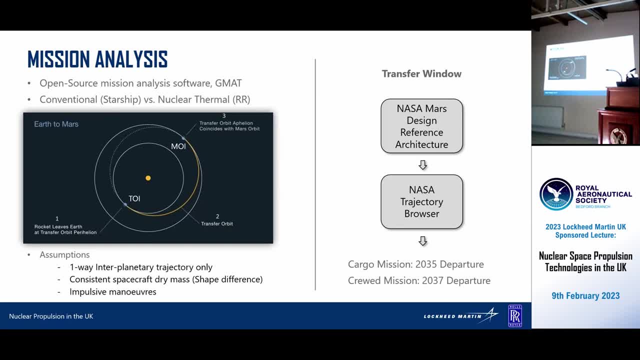 most efficient time to leave earth to get that really nice trajectory up to mars, and we resulted in a cargo mission of 2035 and a crude mission of 2037.. so typically you get these kind of two-year gaps just because the way the orbits work um two years is typically the. the difference between 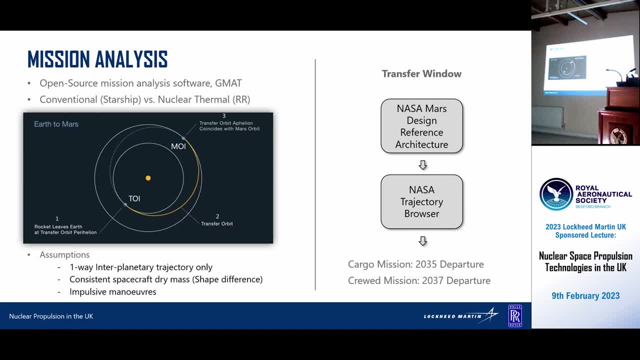 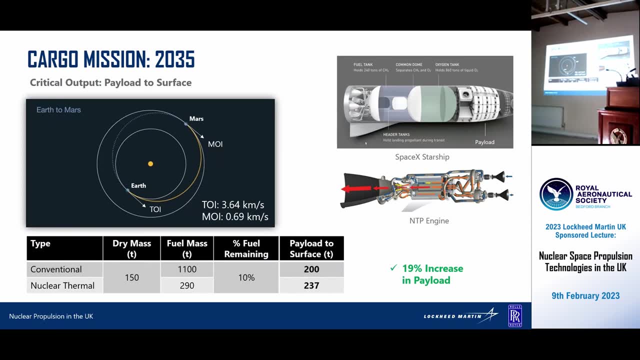 useful um trajectories, so running all of that information into our software. um, we're looking at cargo mission in 2035, so there's a few assumptions that we've made here. so, as i said, dry mass is the same. the starship with all of its fuel loaded up. 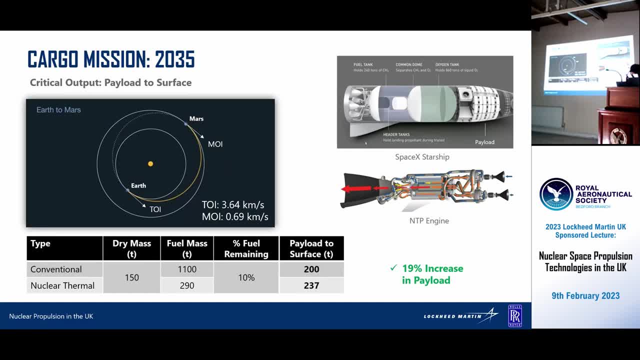 so our assumption basically says: we're going to drain the fuel, drain the ship of all of its fuel that's remaining. we're going to keep that the same, refill it with nuclear thermal fuel, so liquid hydrogen. the comparison between the fuel mass there is massive. so because of that oxidizer, that 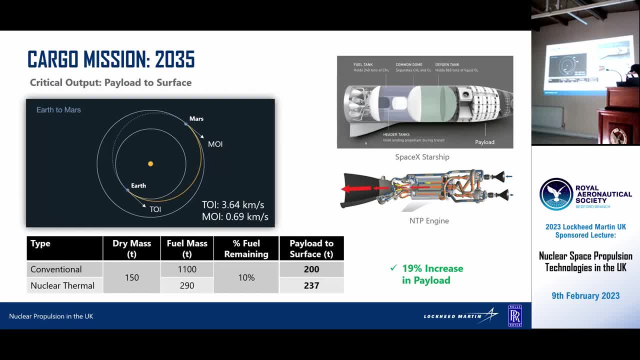 uses up so much volume. we can remove that. fill it all with hydrogen. much lighter fuel gives you a much lower fuel mass. then you can perform your mission. um pairing conventional nuclear, we get a payload surface increase of about 20 with nuclear thermal. so that's without optimizing any of the structure. 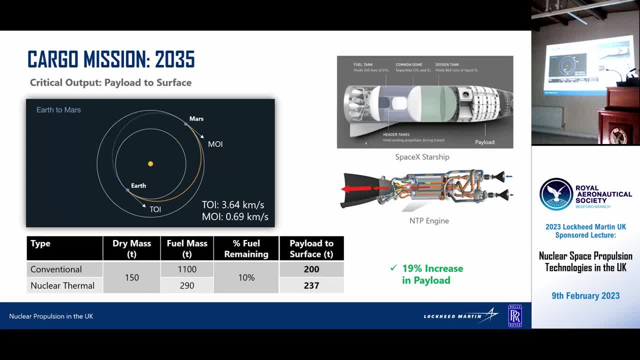 any of the actual design of the spacecraft, you get a pretty significant increase in payload. so then with the crude mission two years later. so we kind of tackled this in a slightly different way, where we make the same assumption about the drive we're going to take 100, pay 100 passengers in both conventional and nuclear thermal. 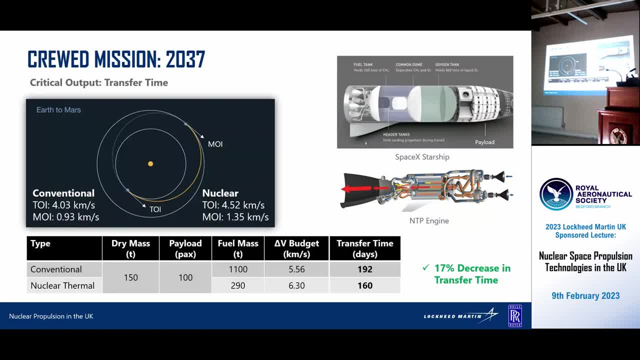 and we're going to take 100 passengers out of these spacefs to turn the payload on and we're going to take 300 passengers in the atmosphere because we're going to tax that fuel mass and we're going to take the fuel mass. we need to keep that fuel mass. the same function about. 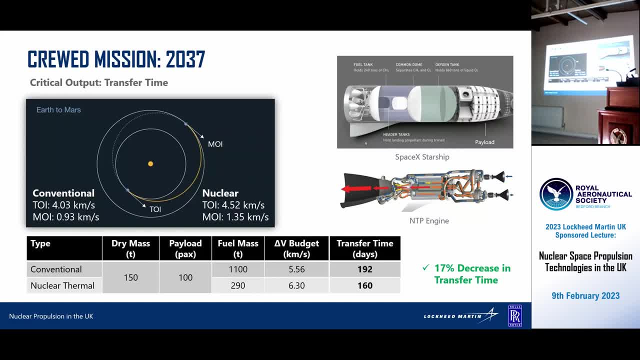 the fuel mass at this time because we want to calculate the maximum velocity change that we can get out of our spacecraft. so running through the numbers, we can see that even with a much smaller fuel mass in nuclear thermal we get an even higher total velocity change, which allows me to 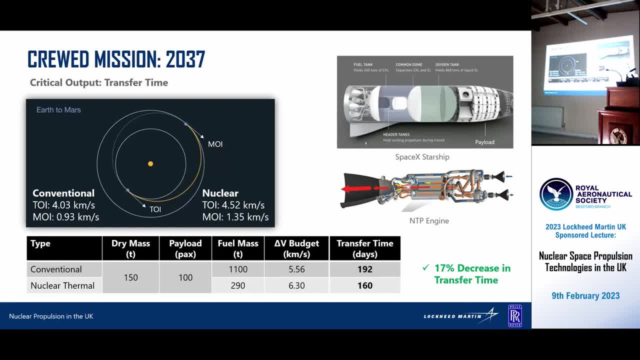 the Martian surface you can still slow down, be captured by the gravity and move much faster. So I think in the conventional case it was around six and a half months, In the nuclear thermal it was about five and a half. And again, that's without optimising anything. 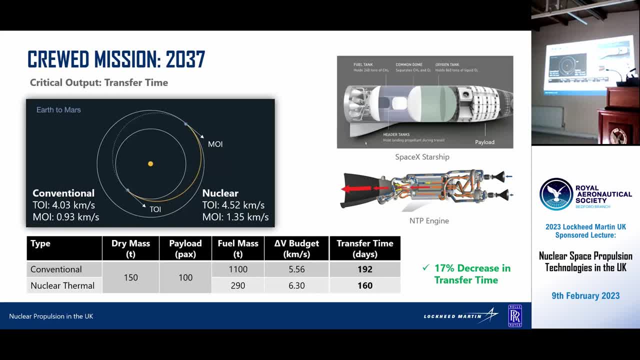 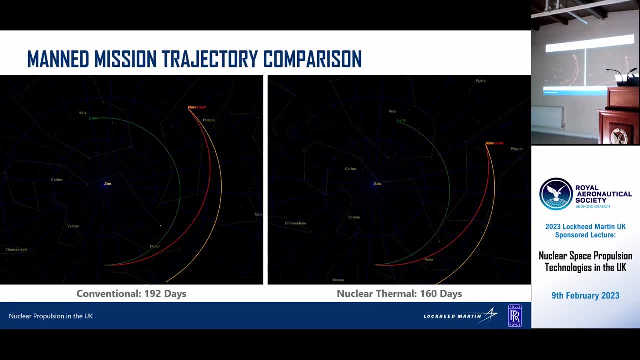 else about the spacecraft itself. it's just comparing fuels. So here's a kind of visualisation of how that looks. So on the left we've got conventional trajectory and on the right we've got nuclear thermal. So you can see that with conventional it takes much longer. 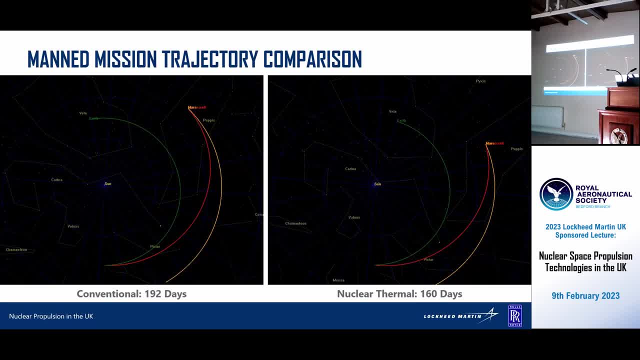 Earth and Mars travel a lot further in that trajectory, Whereas in nuclear thermal we get a much more aggressive trajectory, where we're increasing our radius from the sun a lot quicker, we arrive at the map a lot quicker- And all those good things about reducing radiation. 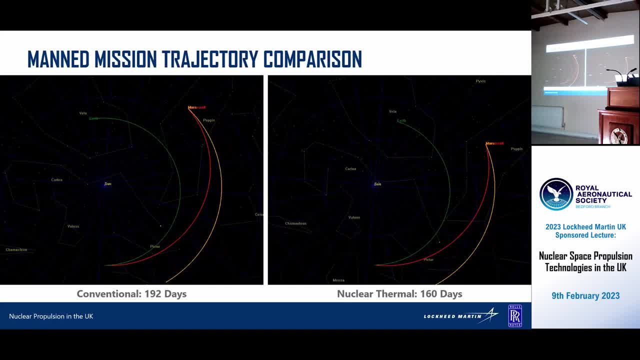 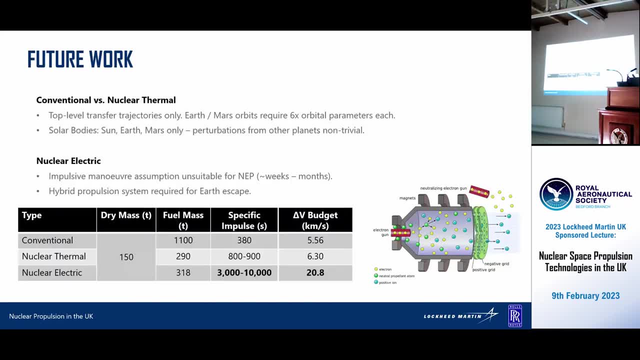 dose. reducing gravity related physiologic effects is beneficial for the passengers. So that was kind of the scope of the technical side of our study. So obviously we've only compared conventional and nuclear thermal If we were to do this in more detail. so we've 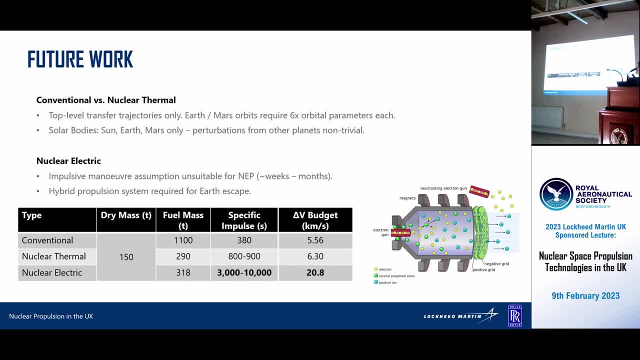 only looked at that step four in that mission profile. In reality, if you were to design a mission like this, you'd have to consider the initial orbit in final orbit around Mars. So that's the scope of the technical side of our study. So that was kind of the scope. 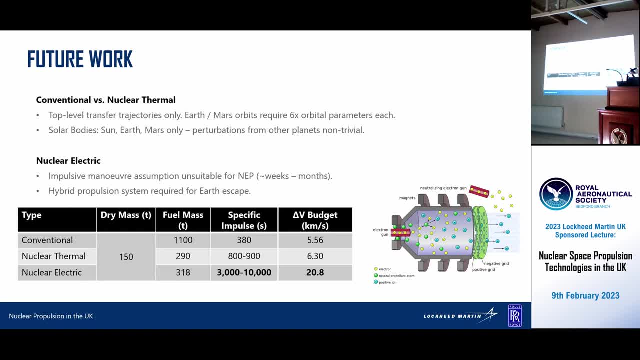 of the technical side of our study. So that was kind of the scope of the technical side of our study. And each of those have six different variables that you'd need to optimize, So in total you'd have 12.. And then you've got that transfer as well, So it's a much more complicated problem. 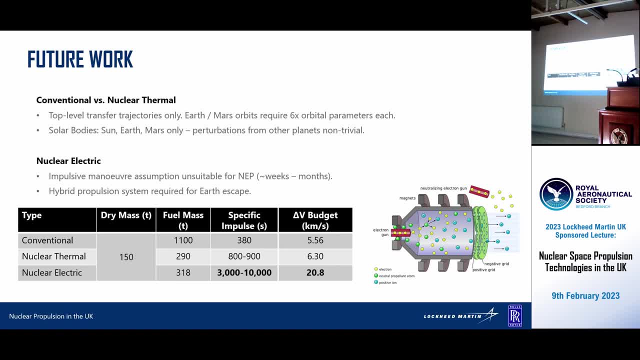 once you start building these additional maneuvers up. So that was out of scope of what we did. If you were to design a proper mission you would do those kind of numbers properly. So the other thing was: in this GMAT code you can kind of decide what. 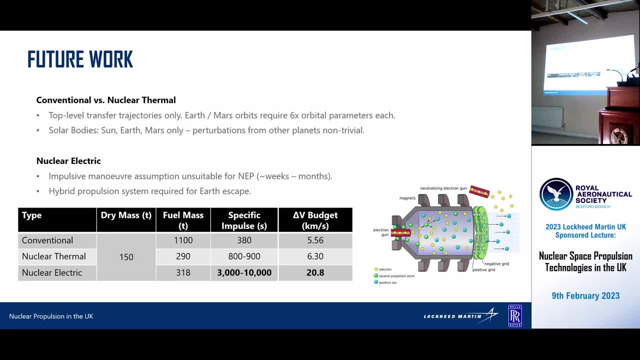 level of complexity you want in terms of which bodies you include in the solar system. So here we only looked at Sun, Earth and Mars, But there's also many other bodies in the solar system that could have their gravitational influence affecting the spacecraft. So if you were again, 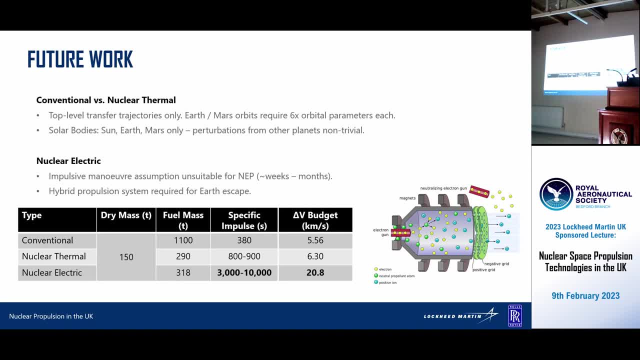 to do this in more detail, then you would include those extra bodies, So then kind of missed out nuclear electric in this. So the reason for that was that assumption about impulsive maneuvers where our velocity change with nuclear electric because you're using, you're basically thrusting your 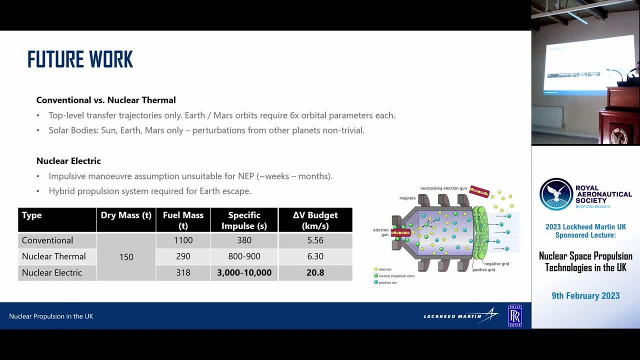 spacecraft for weeks or months. that assumption is no longer valid And it makes the analysis a lot more complicated. when you're trying to burn for a long period of time, change directions, burn for another long period of time and then arrive at Mars at the perfect spot, perfect velocity. So 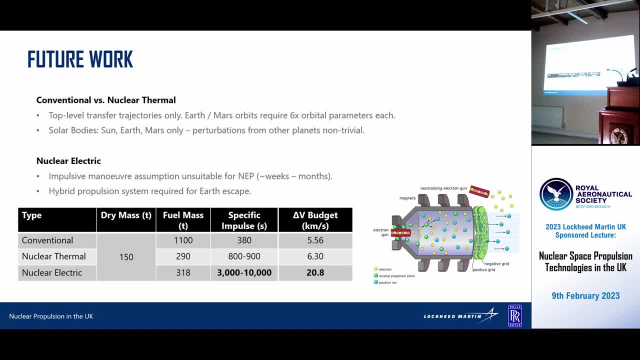 yeah, that takes a lot more computational power than we had. And also, as we were saying, you need a hybrid propulsion system typically, So to escape Earth you probably need a conventional nuclear thermal engine anyway, And then, once you get to, 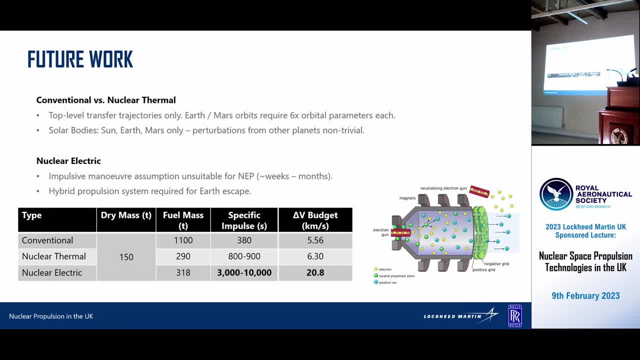 Earth orbit. you replace your second stage with a nuclear, electric. So yeah, that obviously as a whole. that will cause a lot more complexity in your design of the spacecraft, your equations that you're trying to solve, But having looked at some of the numbers you get from, 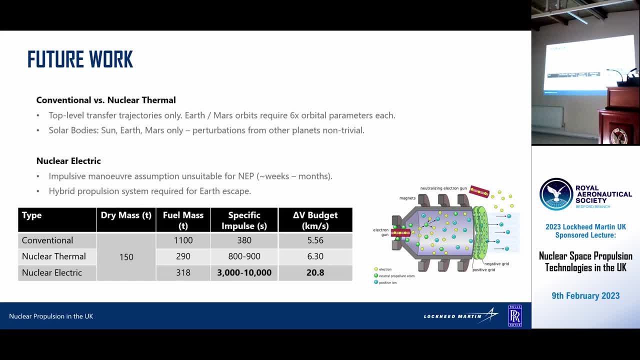 the efficiencies in thrusters, so kind of said, with specific impulse there, which is kind of a measure of how efficient the fuel is and the engine system. typically you get 380 with conventional. You get around double that with nuclear thermal. You get around 10 times with nuclear electric. 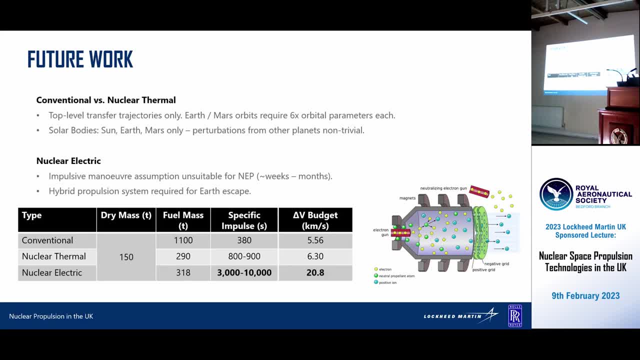 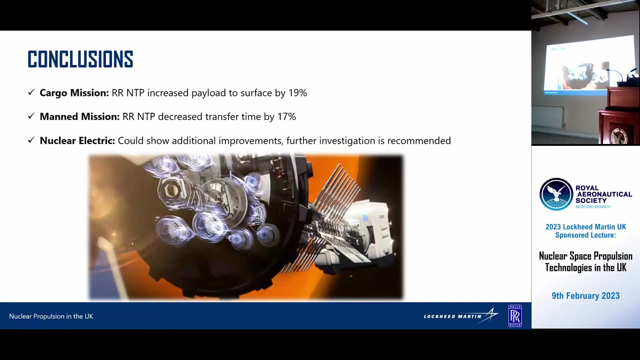 So when we're thinking about the humans on board, we're looking at delta v budgets. change in velocity: you get a slight improvement with nuclear thermal but with nuclear electric you get four times more change in velocity which would significantly decrease your transfer time from earth to mars. so inclusion, kind of already said you can see um sort of improvements. 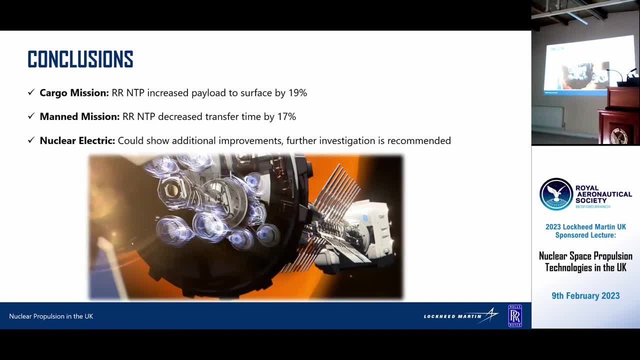 on both cargo missions and manned missions, using rosewood's designed nuclear reactor in the nuclear thermal propulsion system to reduce your payload emission by 20 and you can decrease transfer time in manned missions by 17.. um, obviously, if you're designing a mission properly, increase that's. 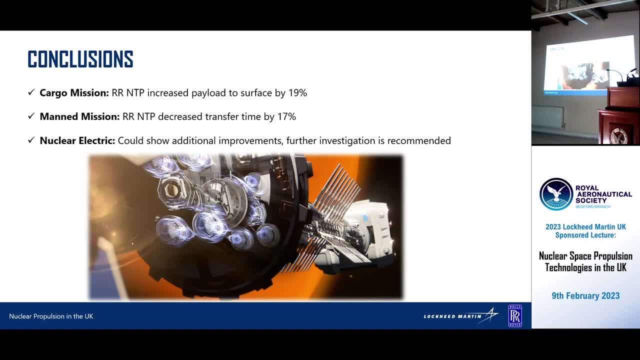 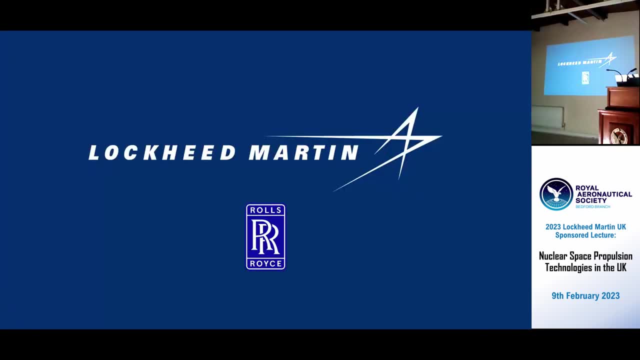 pretty much it, so i'll open the floor to questions. hope you enjoyed it. hope you found it interesting also, uh, any questions in the audience? i'll bring the microphone over. thanks, a couple of questions, um, really on the nuclear power plants, which is not really my field. 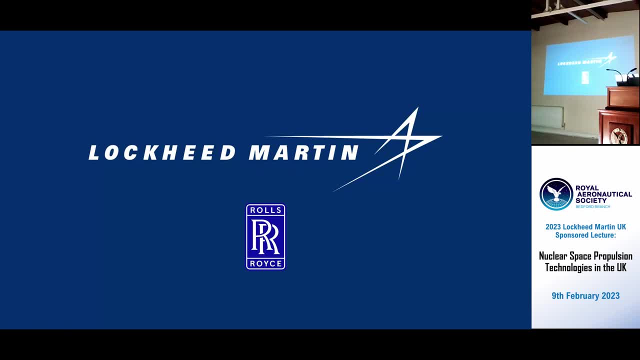 but i get the impression from normal nuclear power plants that these are fairly slow to start up and to shut down. um, you put the control rods in, you know, to mitigate the fusion reaction. then it takes a long time for the thermal mass to decay. so i assume for this that you sort of light the fuse on this rocket and 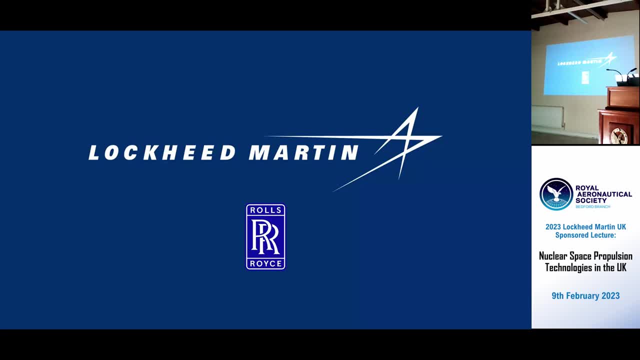 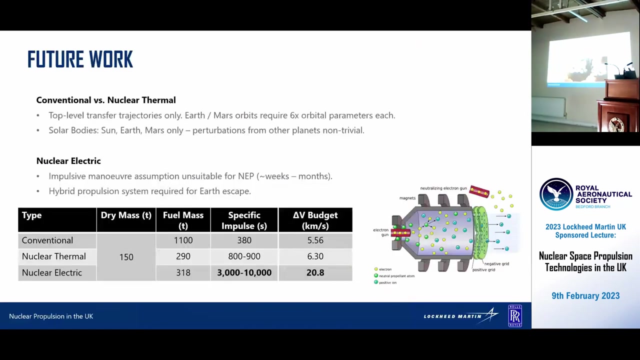 wait a week before you climb into it, yeah, so, um, and how does that work when you're in in flight and you want to do another burn? do you shut it down when you're coasting or uh? yeah, so obviously kind of nuclear, uh, reactor side things was rolls royce's expertise there, so 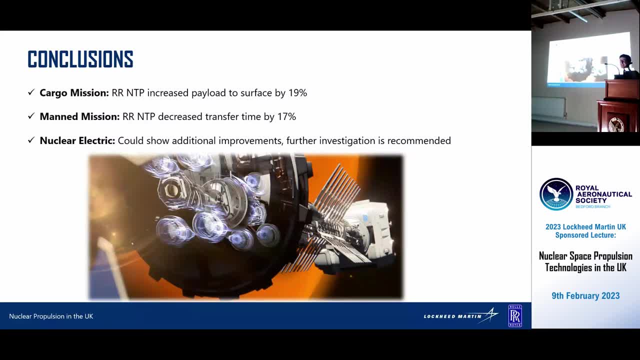 i'll probably give the best answer i can. so what i'd assume: before you launch your spacecraft you would initiate the fusion react- efficient reaction- in the reactor before you launch. so by the time you actually get to launch, your reactor is already producing heat. it's already at the 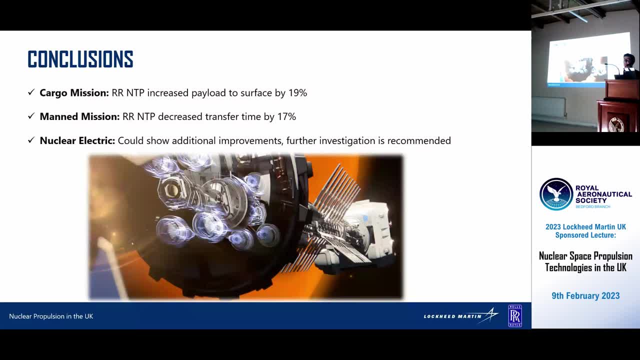 moment you've kind of been in equilibrium with the conditions that you need to be able to pass fuel through um. second question is on: once you get into space, how do you stop, stop the burn and restart it? so i think that kind of comes with the cooling system. so what i'm assuming is that you 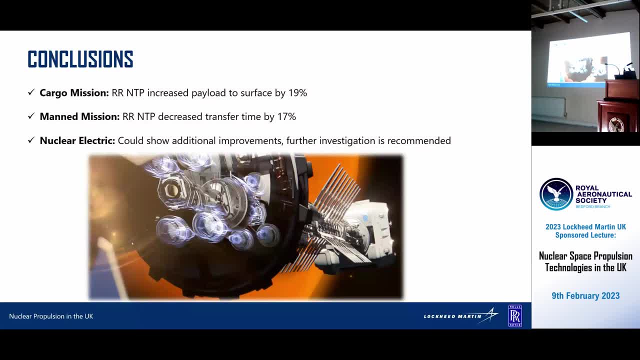 would keep your reactor um doing condition the entire duration of the mission at a constant rate. um, you constantly be rejecting heat while you're traveling to relight your engines. you would then have the right conditions to be able to pass fuel through at any time. so that's probably the best answer i can give without being an expert. right and the 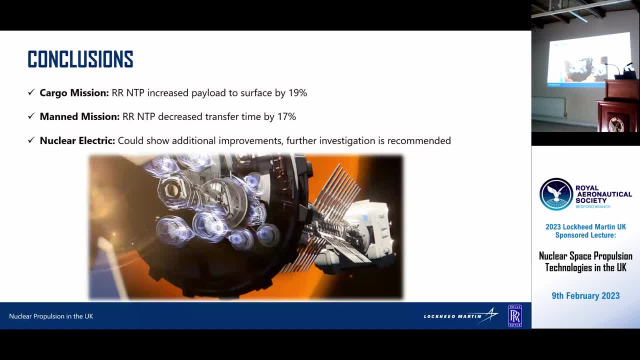 follow-on to that really was the nuclear electric um. you sort of said it was fairly simple, with few floating parts, but my is that if you look at a standard nuclear power station then, yes, there is a big reactor vessel, but then alongside it there are some enormous generators, all of which 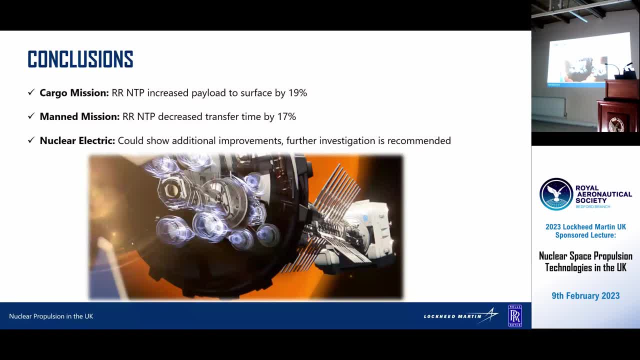 have got great big steel masses hurtling round and round with enormous gyroscopic effects. so with your, how do you generate the electricity? is it a computer? i know that electrical generation technology is what? 150 years old, but it's still got some fairly significant problems with it. 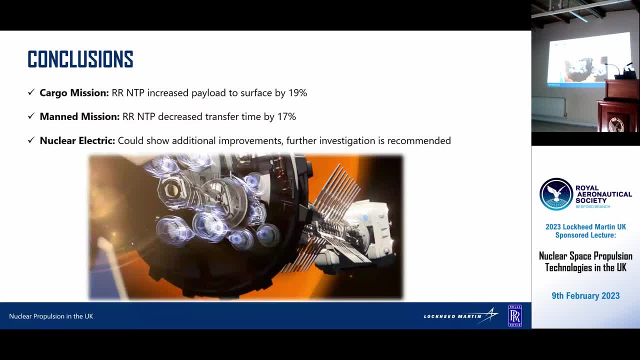 and, of course, working fluids, sodium or water, or so, again, not an expert in nuclear power production, um, i do know there are systems out there that can convert heat to electricity directly. so think about formula one cars. when they do regenerative braking, they convert heat directly to electricity, without the 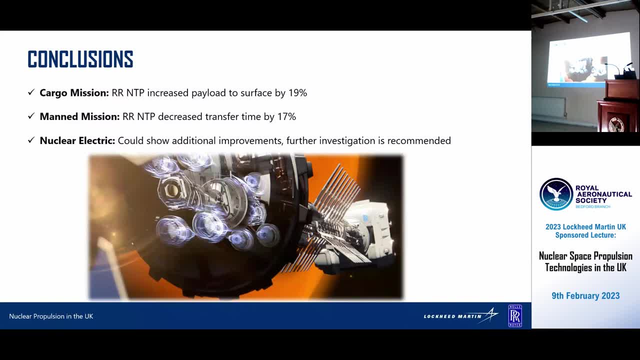 need of a working fluid. i don't know if that creates enough electricity to be able to power a thruster, but i'm assuming there's some clever new technology that has been developed to be able to eliminate a need for- maybe not eliminate working fluids entirely, but be able to generate it in some other form. 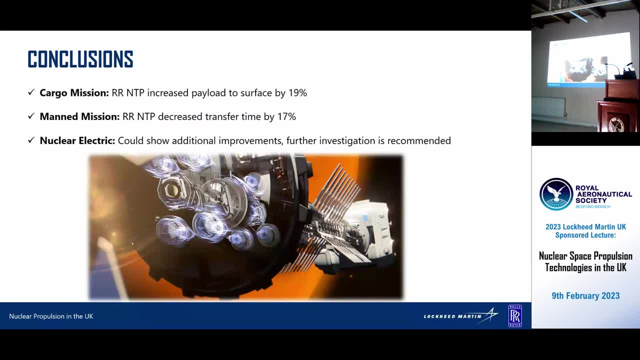 well, um, any other questions in the audience? okay, yeah, thank you for the presentation. um, i was just wondering. you mentioned earlier there was an assumption about um, assuming that the velocity changes instantaneously and as we're looking at the motion systems, where the thrust is becoming lesser and lesser, um, i imagine that assumption makes a 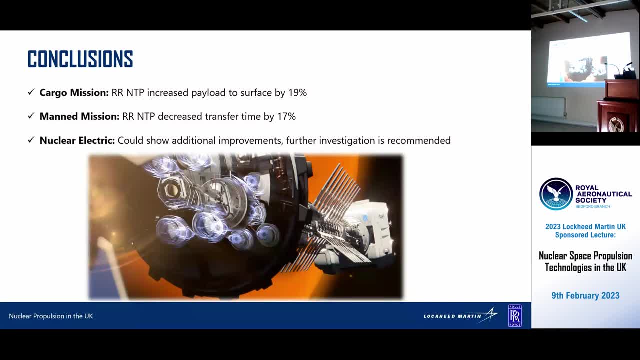 bigger impact in the calculations for the mission, and i'm just wondering um what systems or solutions are in place for readjusting, um the issues of the, the trajectory, i suppose, yeah, third times, um, you see, when you generate, when you create a spacecraft, um you've got some pretty high. 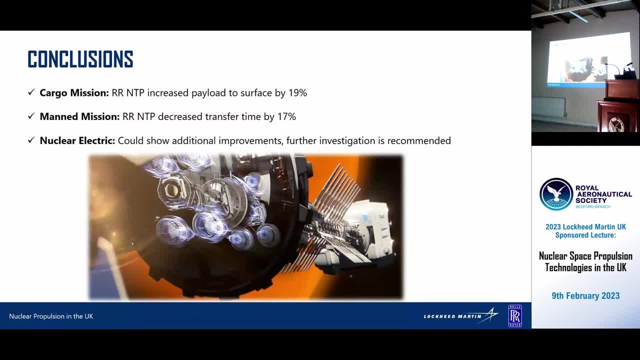 technology systems that deal with calculated projects. um, you've got some pretty high technology systems that deal with calculated projects. um, you've got some pretty high technology systems that deal with calculated trajectories. so with that assumption that we made with the impulsive maneuvers, it just makes the modeling process a lot easier. it is possible to model continuous burns. 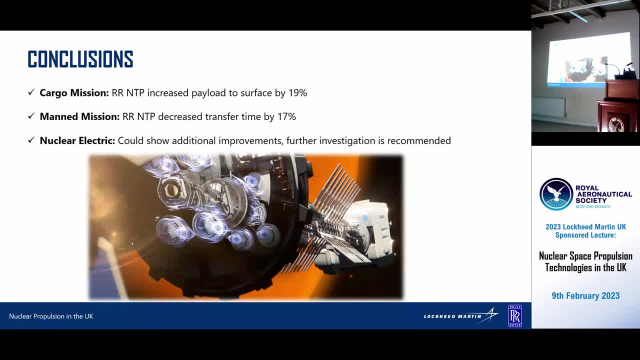 long duration burns. it just takes a lot more time, effort, computing power to do so. so i know there's electric propulsion systems of satellites. so a lot of time when a satellite's in orbit it gets bombarded with solar radiation which decays the orbit. there's also very low. pressure gases up in the in space. so if the orbit is quite close to the atmosphere you do get some drag which kind of decays the orbit as well. so they do use electric propulsion on satellites to boost the orbit where you burn your engine for a long period of time. 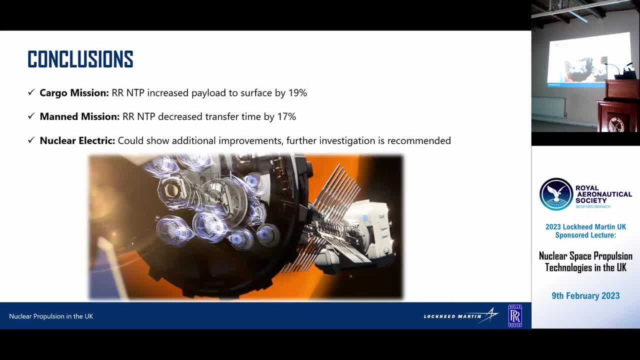 to get back to the position that you want your satellite to be in. so that's kind of what we're going to look at in the next few slides. um, so that there are systems out there actually do these kinds of calculations, and obviously you plan your mission in advance to be able to do those kind of things. so 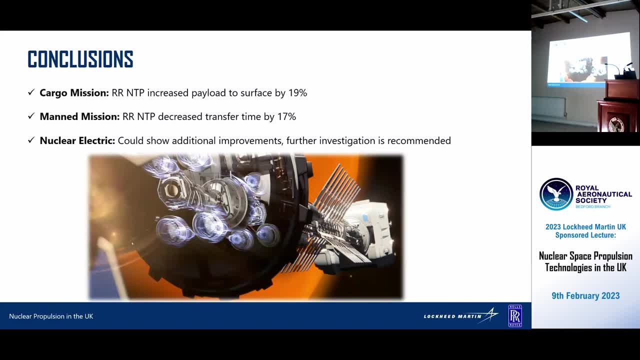 yeah, i mean, i've never done one myself. um, one of the reasons i recommended it the future is because i think it's a really difficult problem and especially for these planetary trajectories where you've got the earth moving, mars moving at a different speed. you need to really get that perfect. 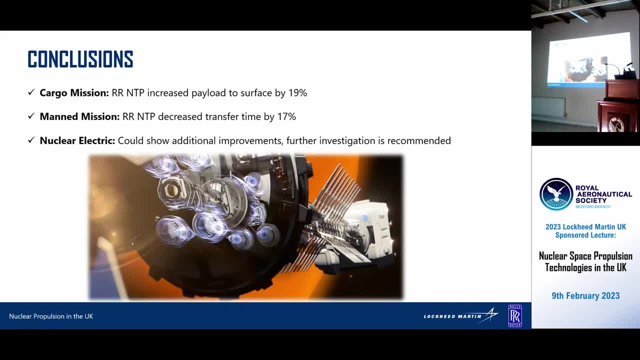 position and velocity to be able to meet mars at the right time. so it's a really difficult problem, but people have solved it before, so no questions. so i've got a quick question for myself actually. um, so i sort of noticed a lot of the sort of things you used to sort of develop the mission. 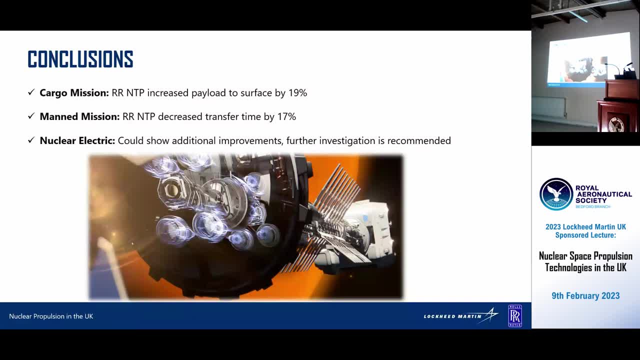 architecture. were you surprised at the amount of uh, open source and readily available materials that allowed you to sort of develop and mission architectures? nasa are really good at having things open source, so using their trajectory browser, using their mars mission architecture- still open source stuff. they they're really good at putting things out publicly, so i would say i was surprised. 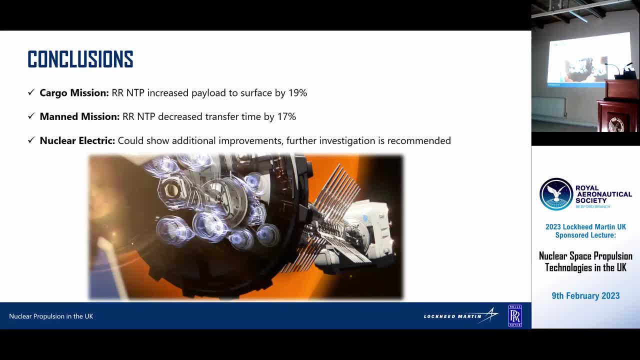 i have used nasa documents, nasa software before, but yeah, i mean you can find a lot out on the internet these days. and yeah, i guess rolls royce was a great help with that as well, because they've been researching these kind of things for decades, so they pointed us in the right direction. 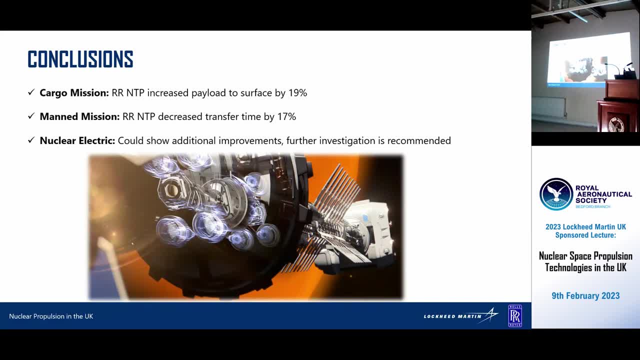 really early on, which allowed us to take it as far as we we did. yeah, i'd say i was fantastic. thank you very much. um, we've got a couple of questions actually in the chat as well, so i'm gonna quickly bring those up. so we've got a question from uh student s. okay, um, hi, uh, my question uh to. 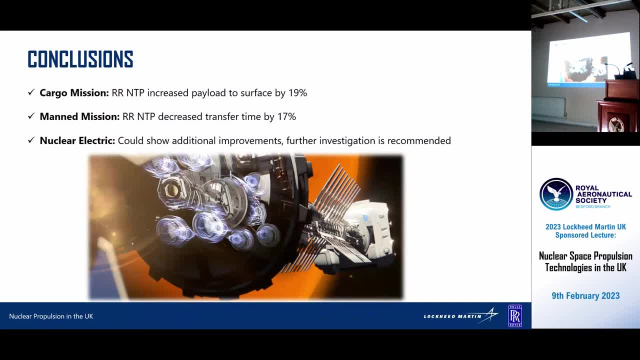 sam is: have nuclear actors considered for long-term deployment missions, such as the new space station? considering iss is scheduled to retire in 2030.. so mentioned, basex got contract to develop their starship to transport nasa astronauts lunar surface as part of those artemis missions. the latter ones are: 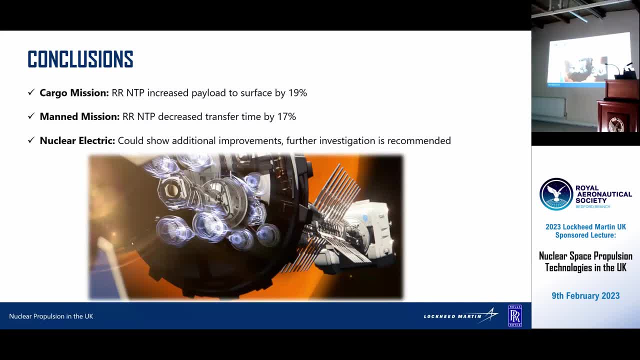 to develop something called the lunar gateway, which is a space station that's going to orbit around the moon. so we're kind of moving from having our astronauts within 400 miles of earth in the iss, to having them permanently stationed on another solar, solar body. the benefits of having 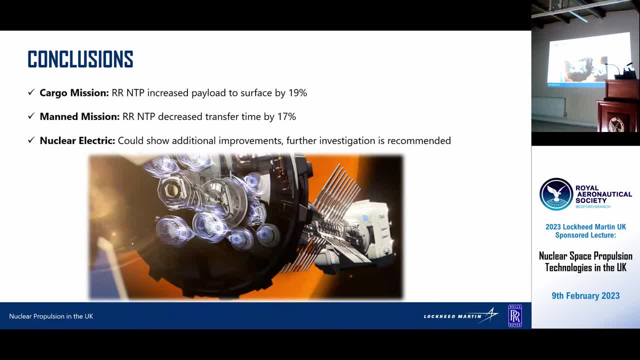 space vacation orbiting the moon is, it's a good stepping stone to mars. so once we have an established base on mars, an established space station orbiting- sorry- the moon, uh, we'll be able to send space graphs to dock with the lunar gateway, refuel one step to the moon gateway. there's very little gravity to escape. 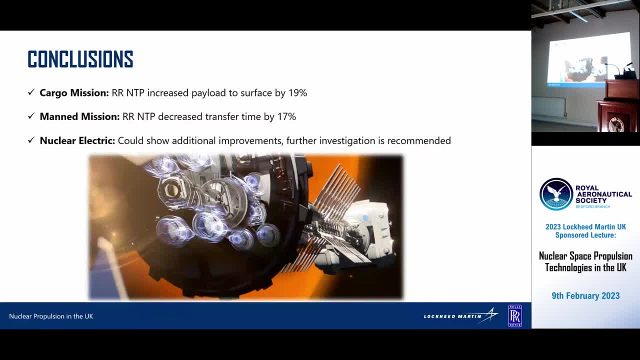 um the moon's orbit. so it makes it much easier to then go on to mars in the future. so yeah, i guess that answers the question. excellent, thanks, um. there's a two more questions in the chat and then we'll hand over to oliver um, so there's two questions from a dominic m. 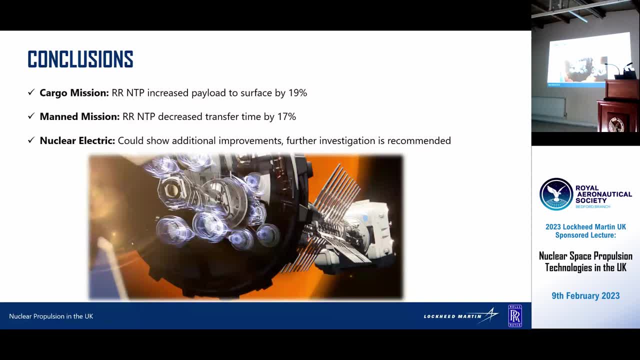 with nuclear systems you save weight on oxidizer. but how does the weight of the reactant cooling systems compare to the weight of the oxidizer? i know a good question. you get a mass saving from there. but then i also mentioned you need things like disc shields. you need that. 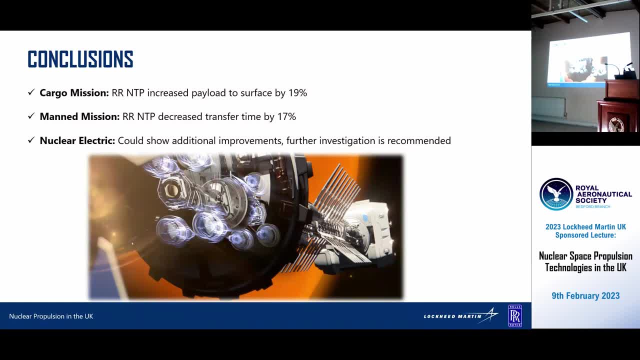 that long structure to separate your engine from your passengers. you need all the cooling systems. typically, you need a fluid to work those cooling systems to reject that heat. so, um, yeah, there is a trade-off. i haven't been able to quantify it in this study, um, but that's one of the things that robert's always really trying to push at the moment is. 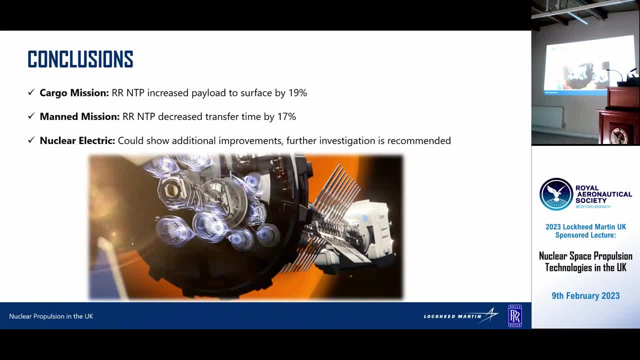 how do these two larger systems compare and can we get as much benefit as we think we can by assuming that that dry mass is the same? excellent and uh. the second question from dominic m is: there's a high failure rate of rockets. how do you mitigate the risk of having a nuclear material on rockets? 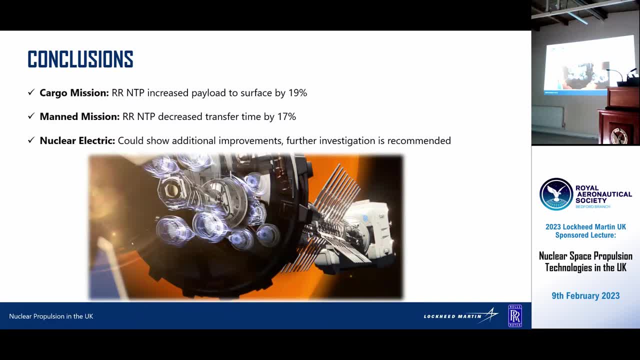 that crash. so that's probably going to be a little bit of a challenge for you to answer that question. tie into some of your experience in hypersonics. reach back to the nerva program. so this was nasa's program to develop a bit of ground. 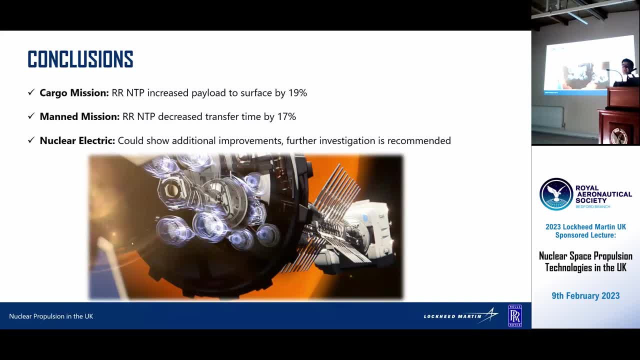 concept of a nuclear thermal. so typically in the engineering process you don't just design something, strap it to a rocket and launch it straight into space. you design subsystems, components at a very low level, testing in isolation, build confidence that they do what they are supposed to do, and then you build. 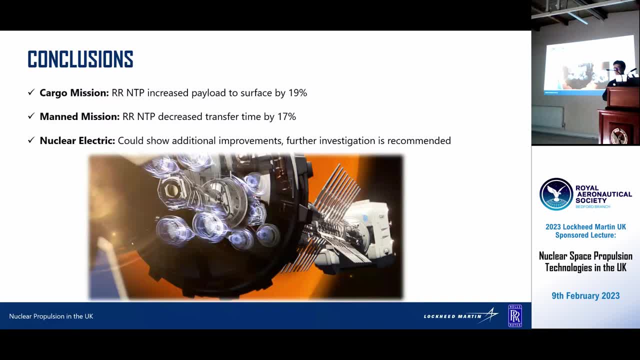 up the complexity of what you're testing. so in the case of this example, um, yeah, obviously you test all the components and then do ground testing, like the nerve- the program was supposed to be doing it- and then you can. then, once you're confident your momentum is safe enough, it's. 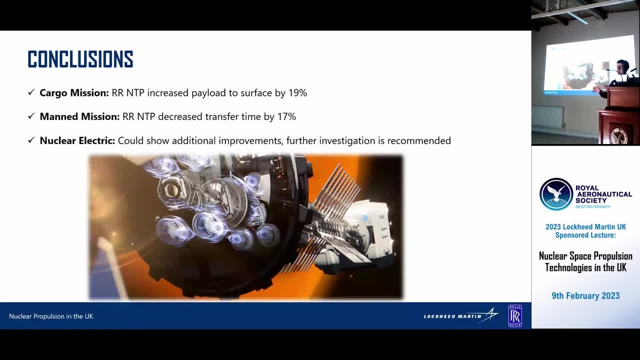 had enough test runs, you're confident in the performance, you're confident in the safety mechanisms around the way it operates. then you can integrate it with the rest of the spacecraft, which will undergo its own testing in isolation, and then you'll have a much more confidence that. 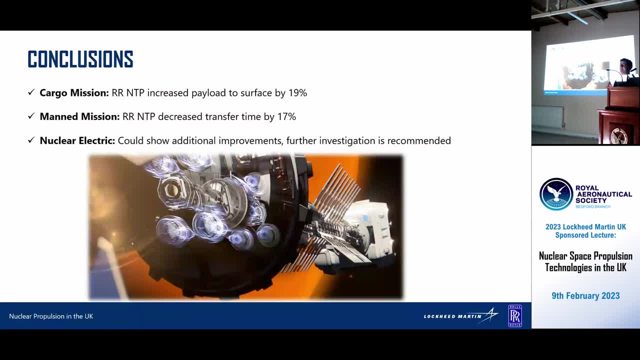 you'll be able to launch successfully. So kind of on the flip side to that, one of the things I did the previous year as part of the PONE conference is look into the policy around launching materials into space. So there's a lot of challenges with policy. so 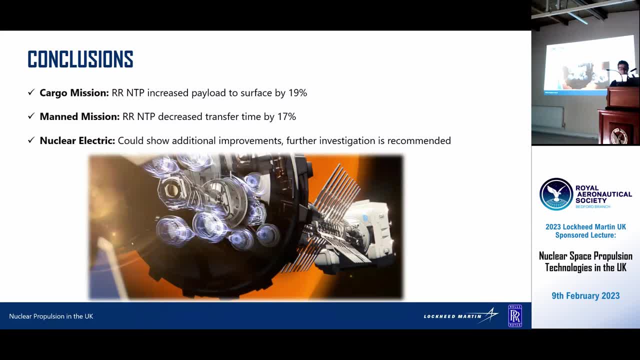 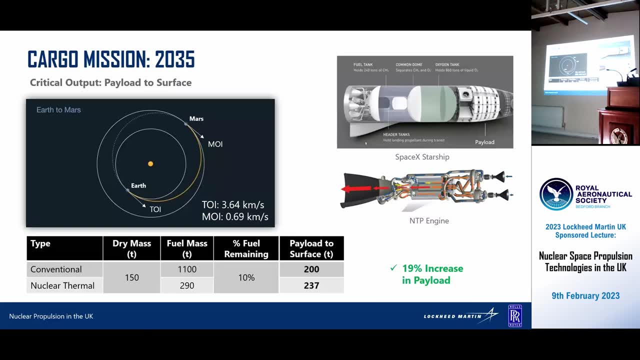 thinking about a company like SpaceX. eventually they're going to be a global company, have sites all around the world and one of the issues is transferring materials into space across borders. So typically all of the nuclear material that's been sent to space previously has 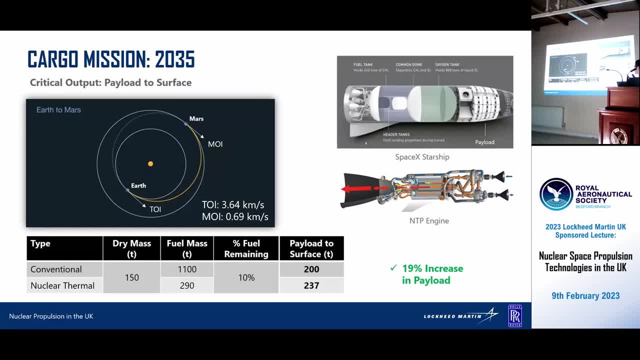 been sent by governments, so NASA, Roscosmos, Chinese Space Agency, etc. Now that we're getting commercial companies to send spacecraft with nuclear materials into space, it becomes much more difficult to legislate that. So transferring materials across borders, purchasing. 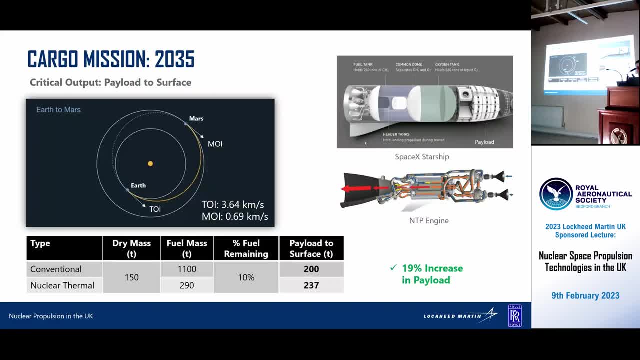 the material. launching nuclear material historically has been purely government-based. You know, when you launch the Mars rover, for example, that has a nuclear power source on it and you need the president's permission to be able to launch that. So it goes right the way up to the leaders of the country. 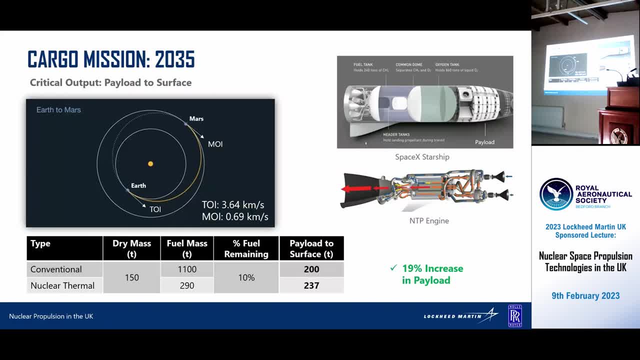 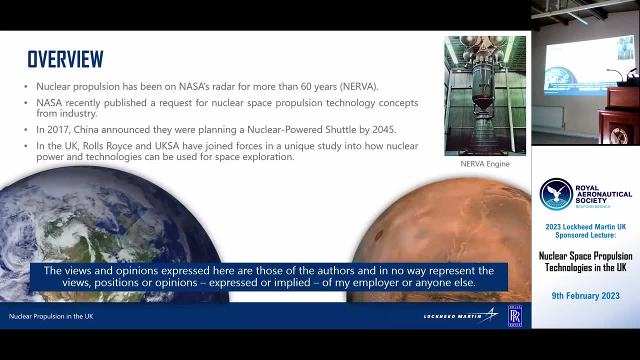 The legislation around companies is very immature. So alongside with this technology development, there has to be a lot of policy development as well to be able to actually make this a reality. so yeah, it's an interesting question. My question kind of follows that in terms of safety, but rather than safety in terms 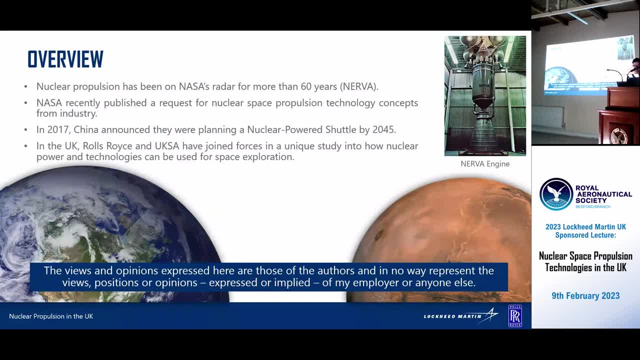 of a rocket launch going down. it's more the safety to the crew when they're in transit. I know we're not talking about nuclear power generation here, we're talking about nuclear propulsion. but when I think of examples and nuclear aircraft carriers and certainly nuclear 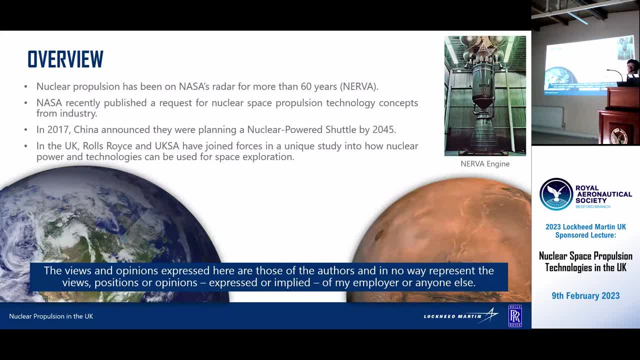 submarines, where there have been tragic incidents in the past, where things have gone wrong and the crew have been exposed to hazardous material. Is that still a risk here, or is it just simply not a fact, because it is propulsion rather than energy generation? But if it is a problem, what has been done to explore that problem? 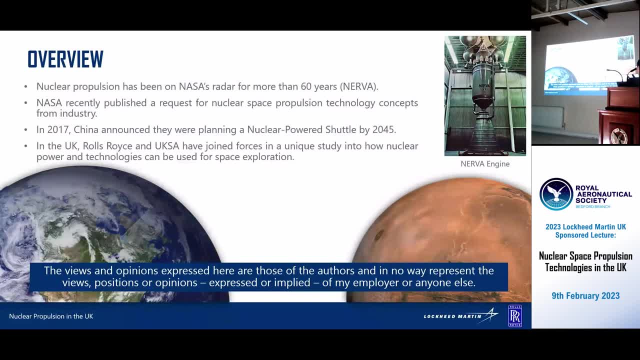 Because I know from previous experience getting safety cases approved and things like this can be an absolute nightmare on programmes. so I appreciate it's a long way off, but I just thought your thoughts were on that It's probably a little bit, maybe too early to be thinking about safety cases in terms. 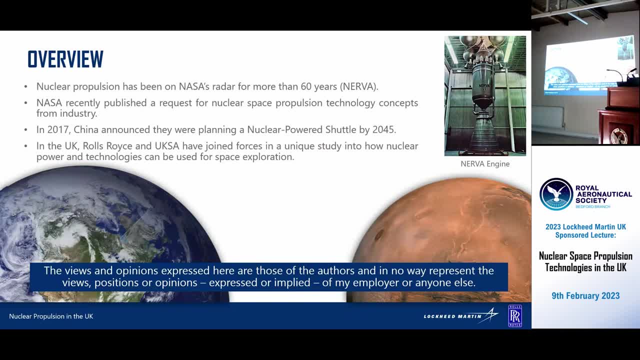 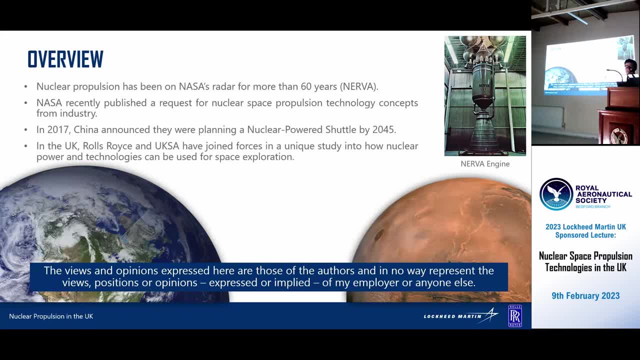 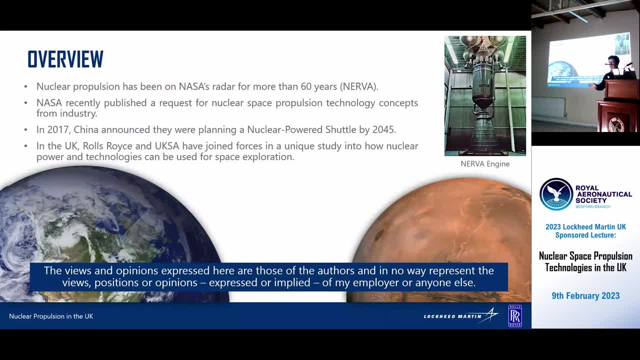 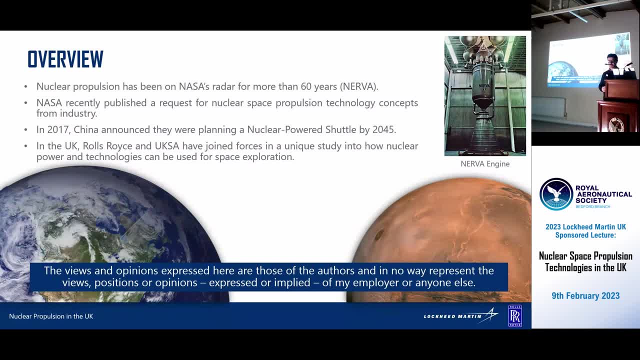 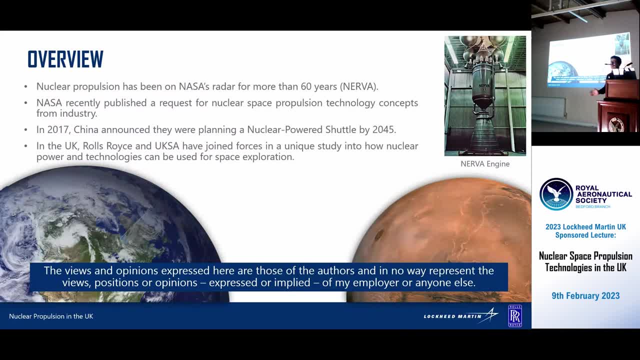 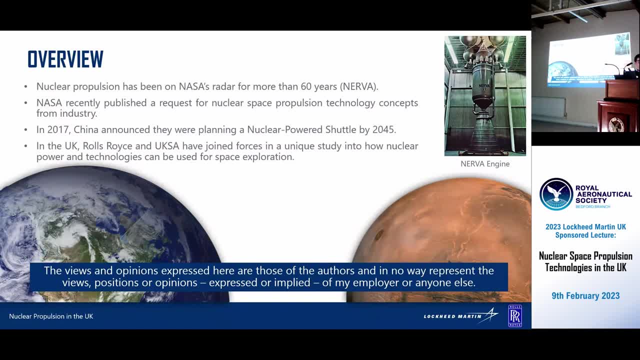 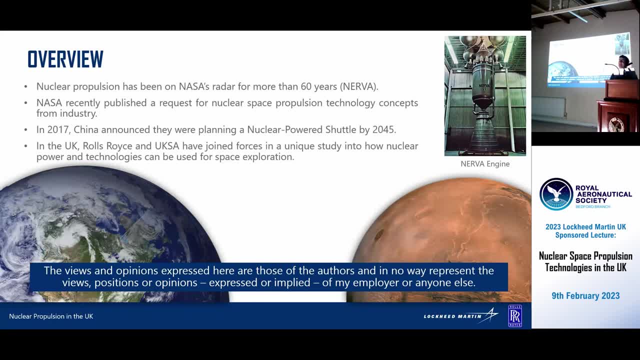 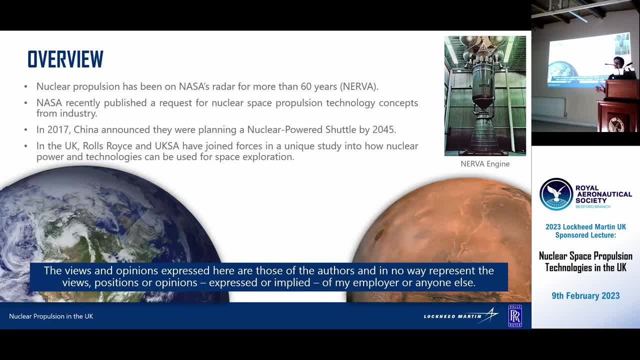 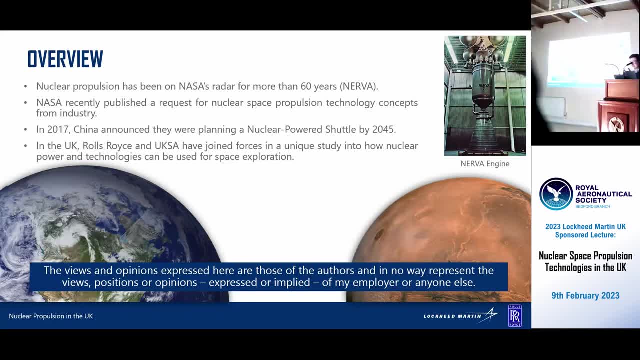 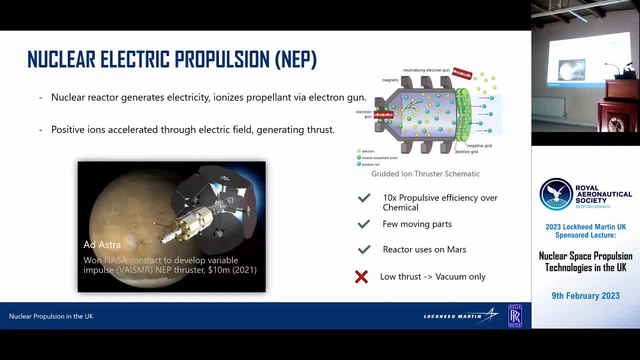 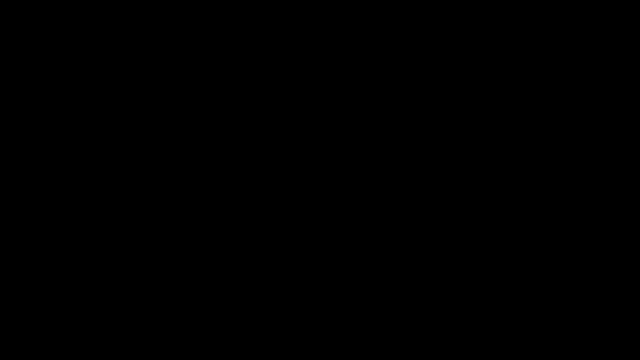 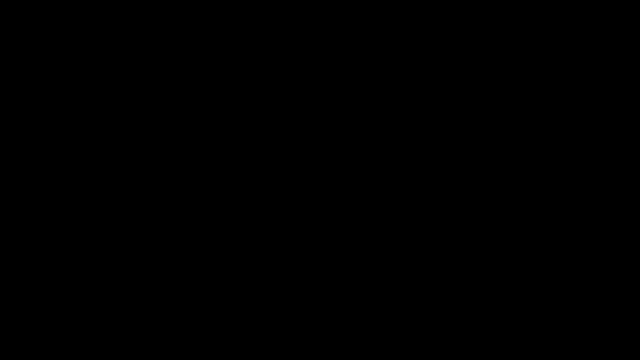 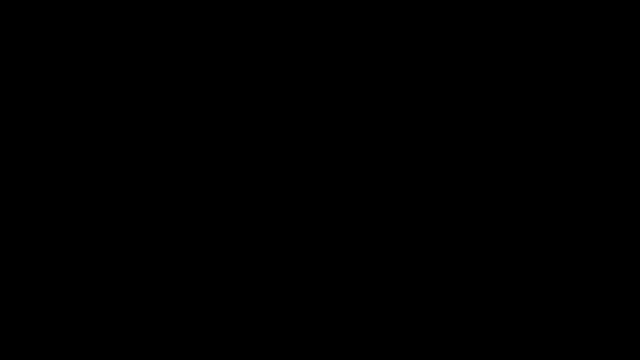 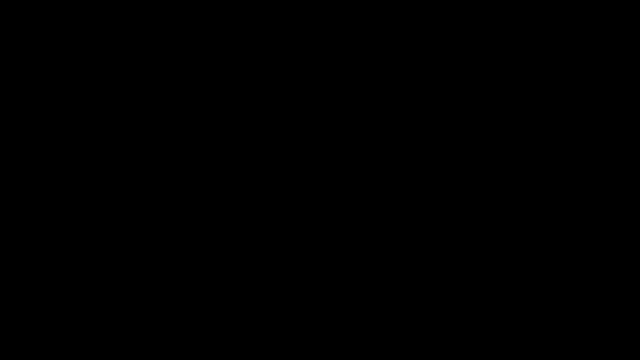 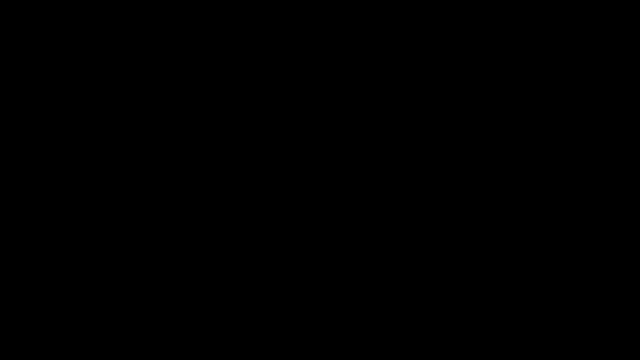 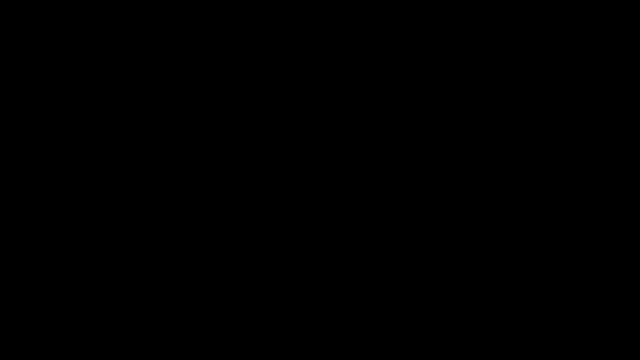 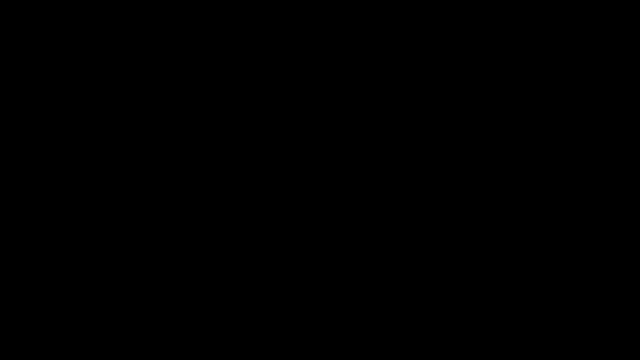 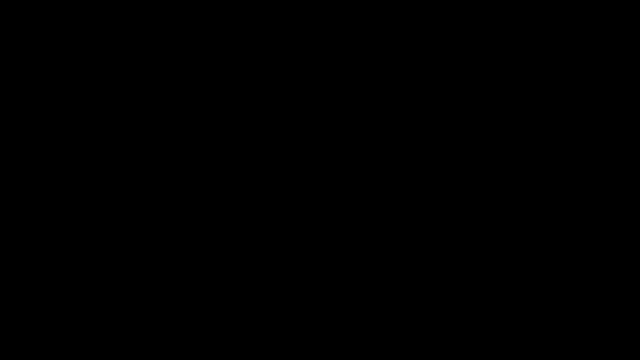 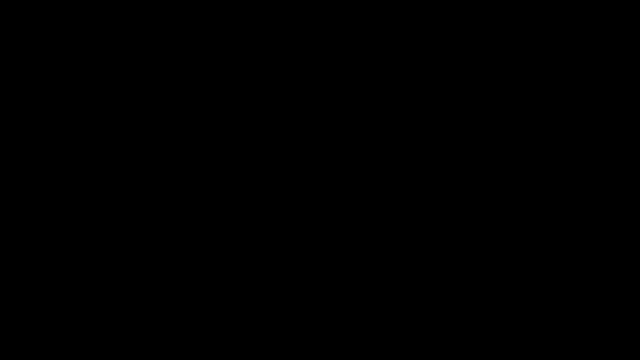 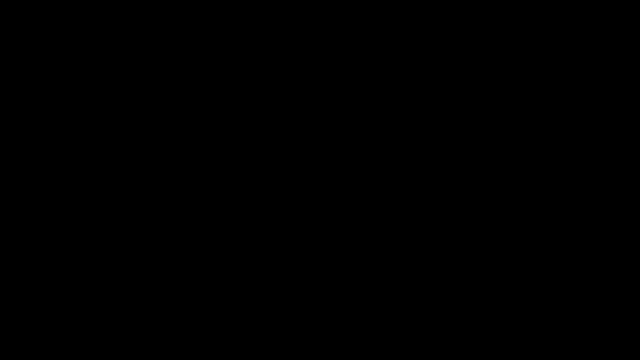 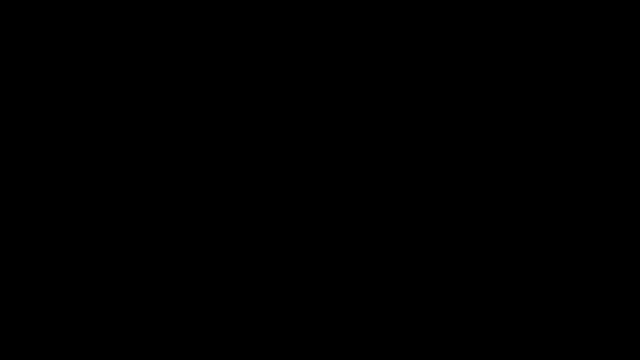 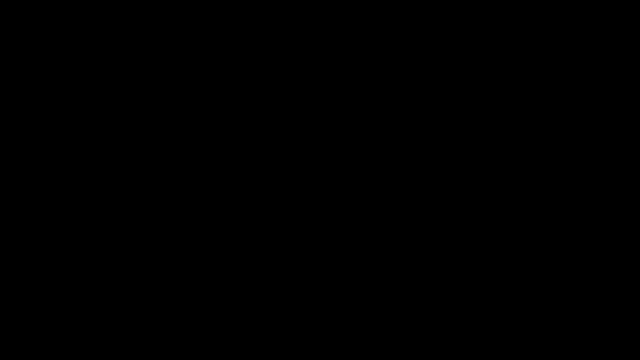 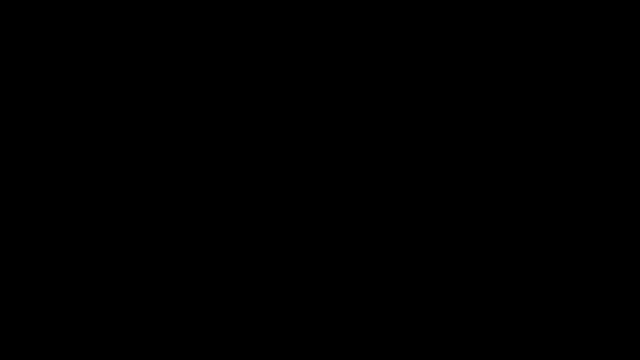 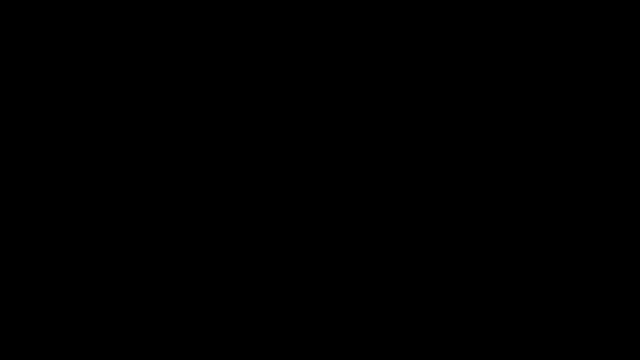 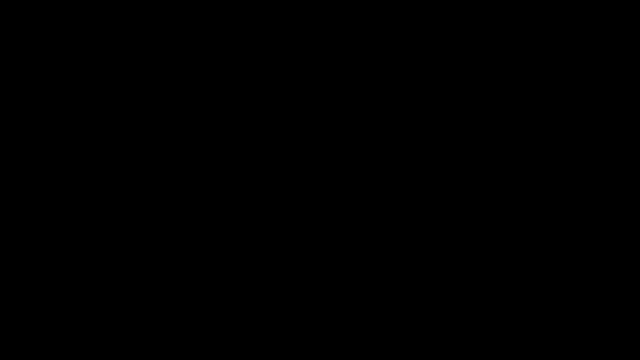 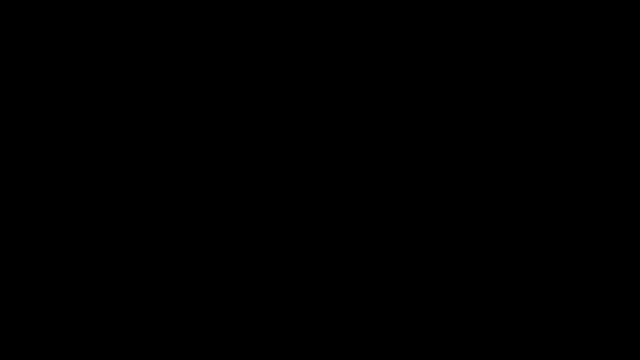 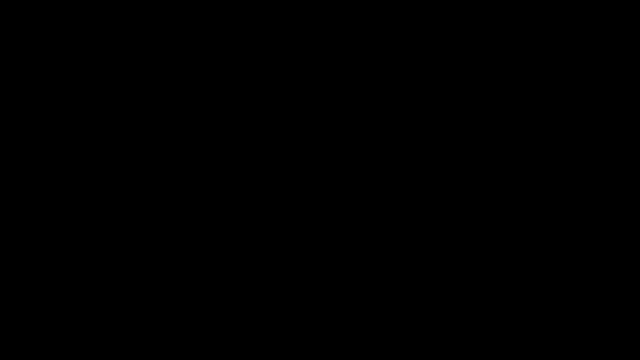 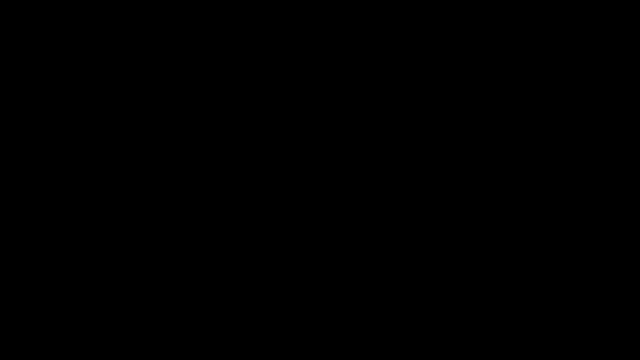 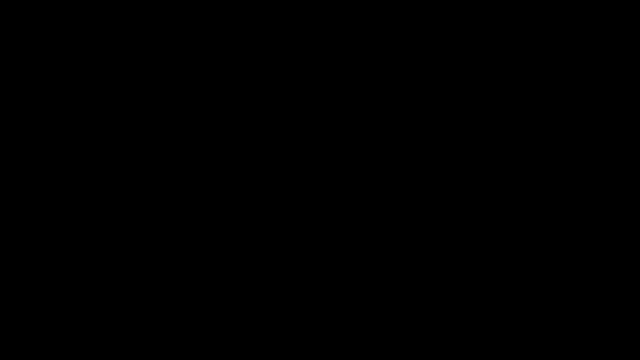 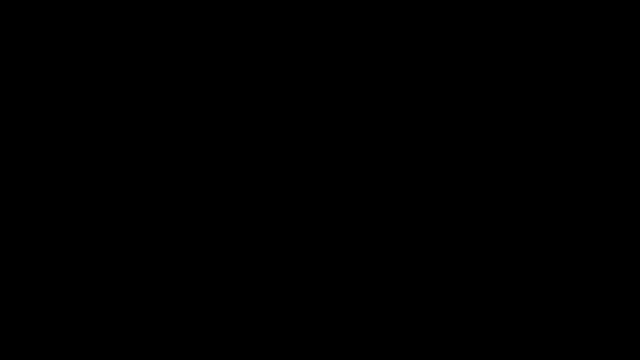 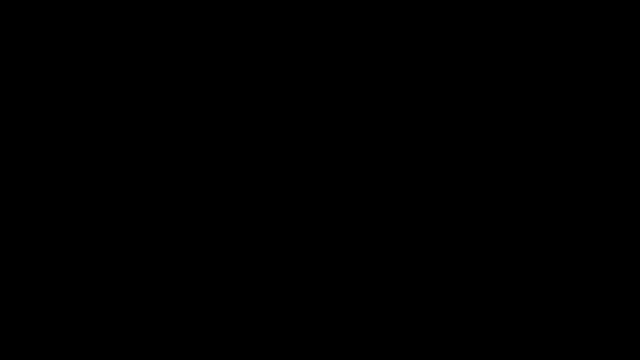 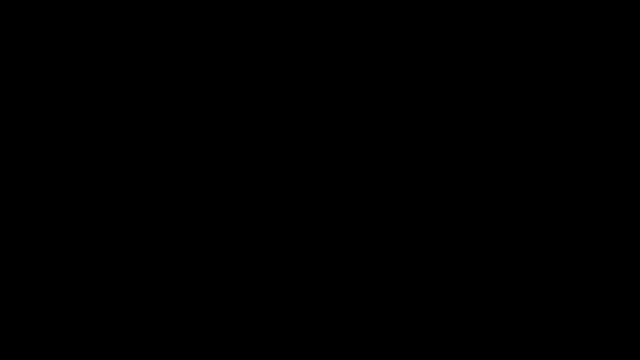 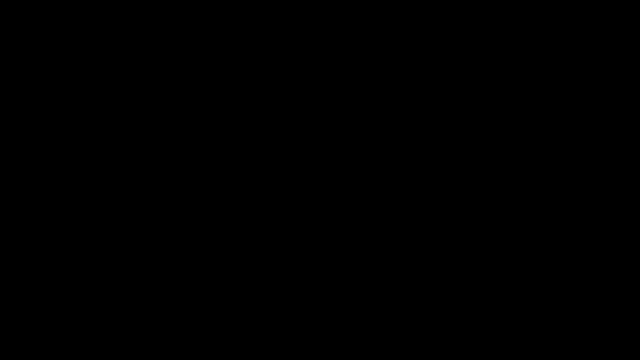 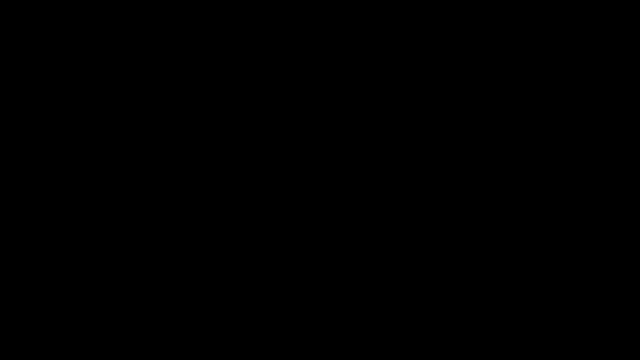 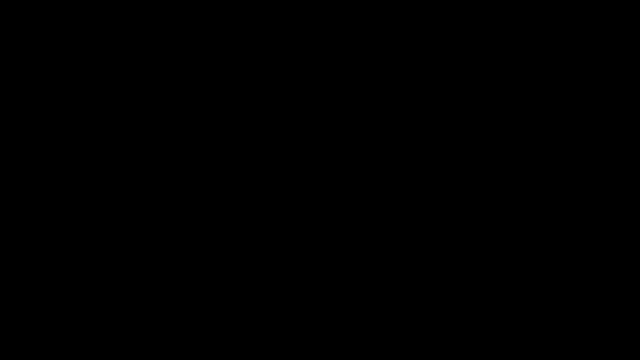 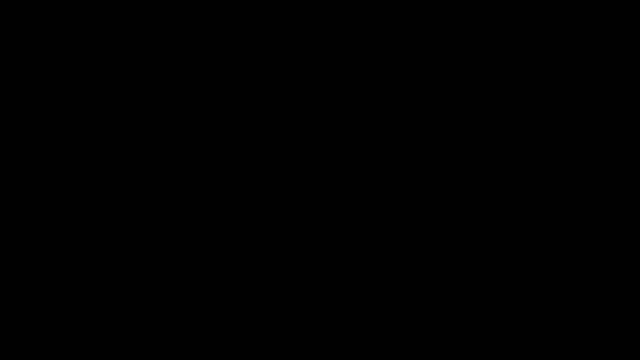 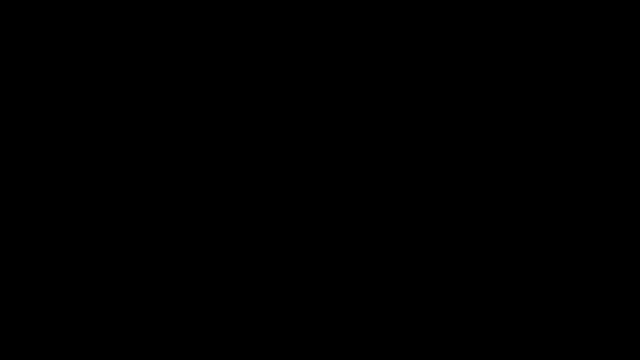 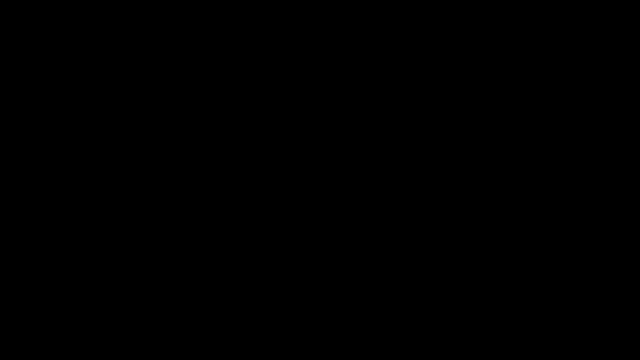 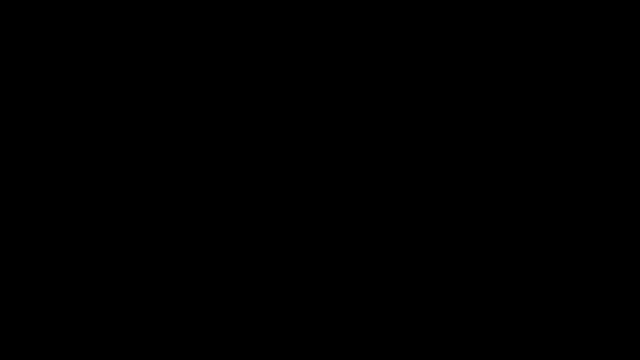 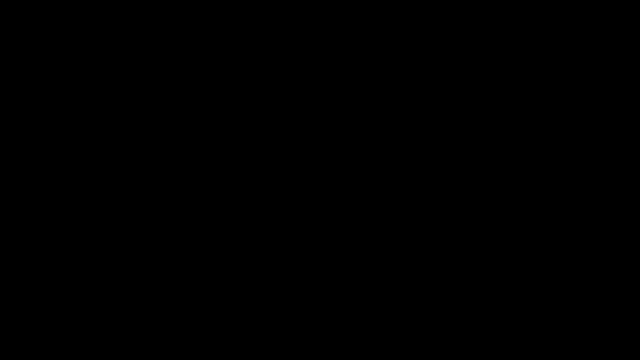 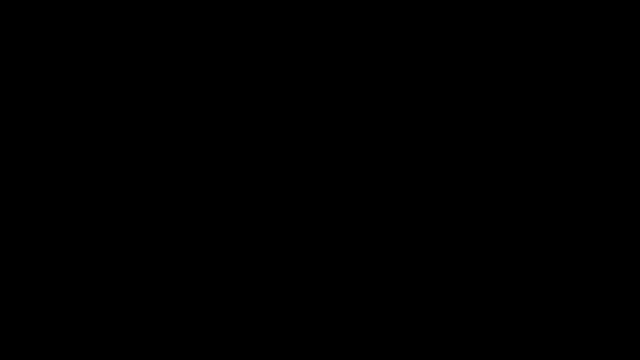 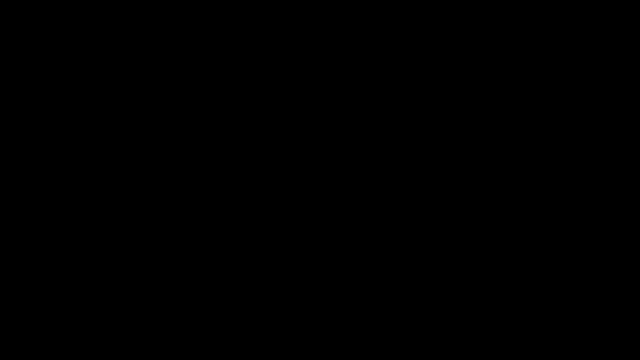 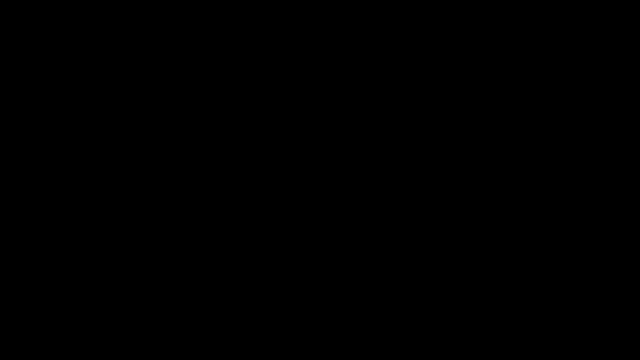 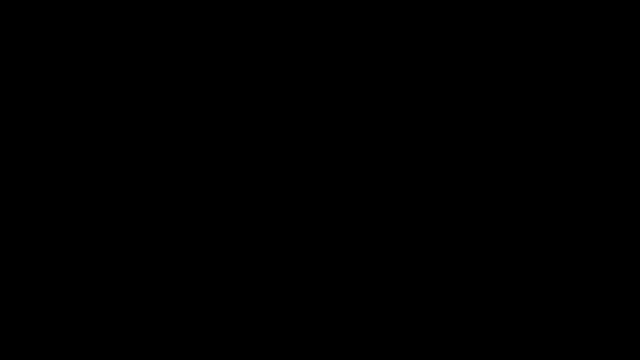 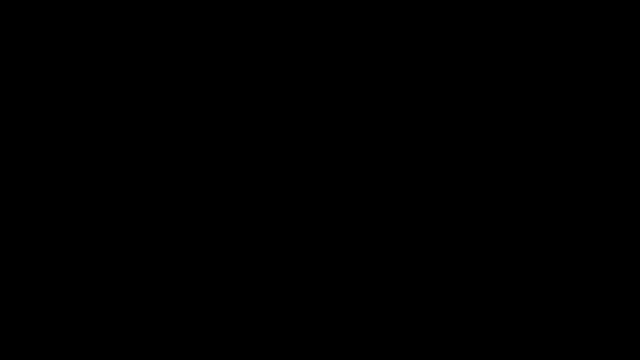 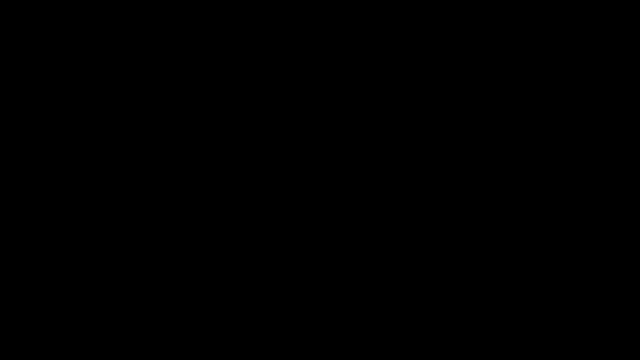 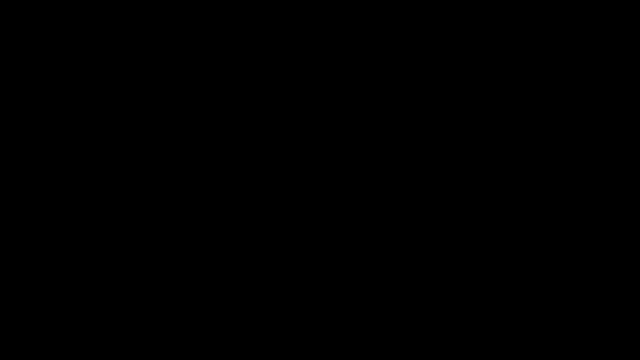 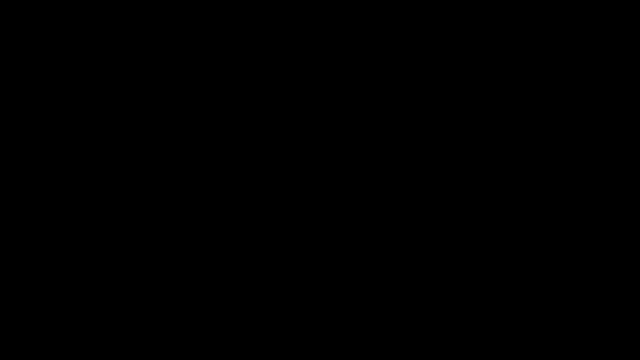 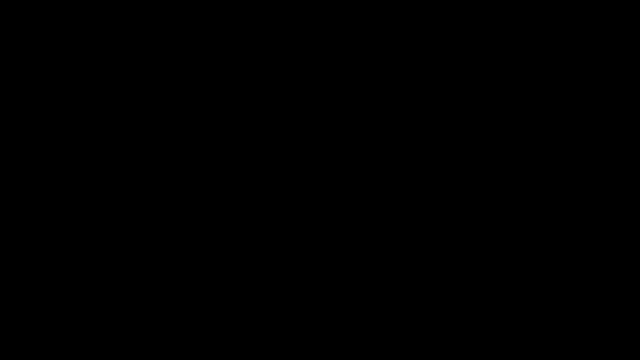 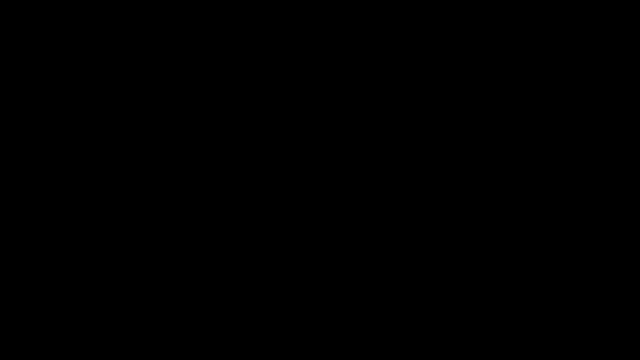 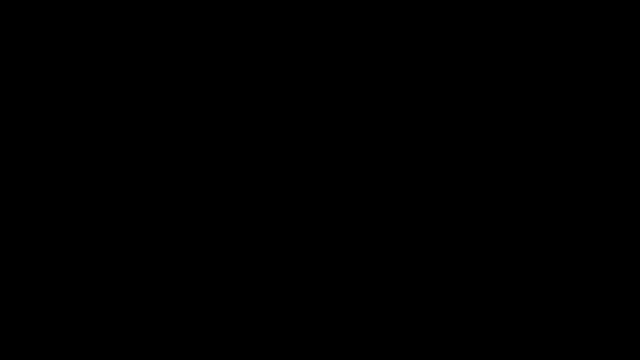 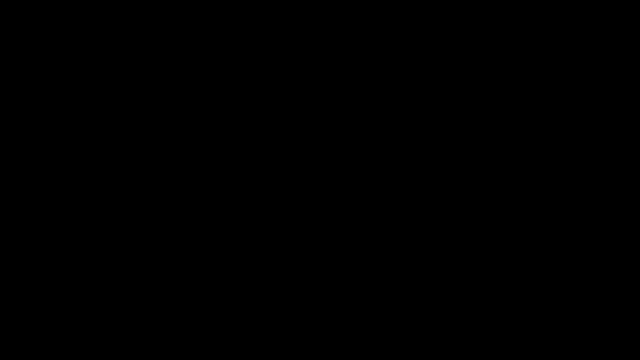 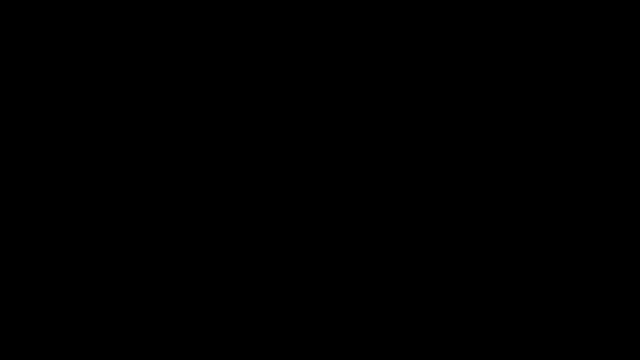 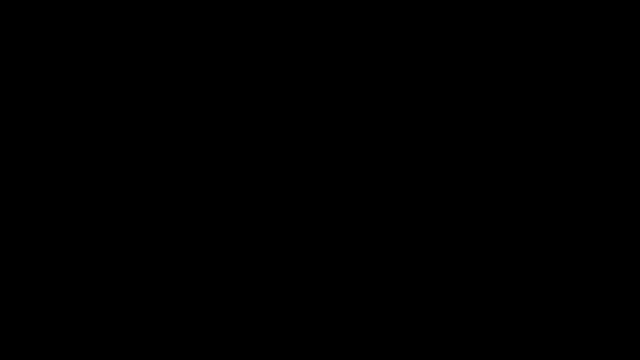